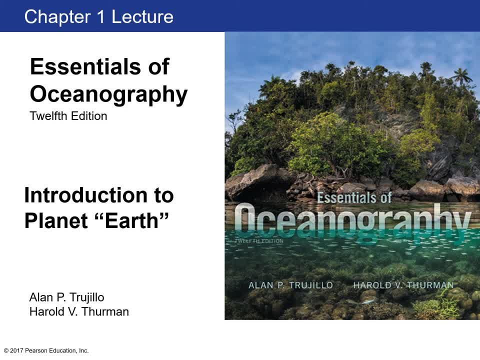 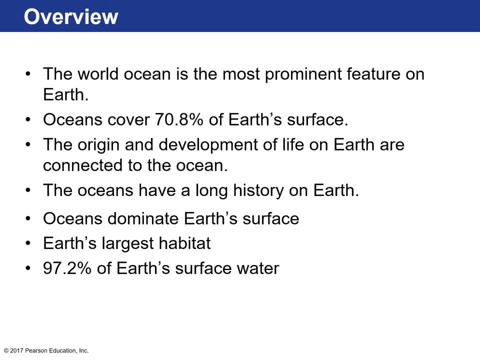 Hello and welcome Oceanography class. This is the first lecture on chapter one, Introduction to Planet Earth. So our world ocean is the most prominent feature of our planet. It covers approximately 71% of the Earth's surface. So if you were kind of a visitor from, 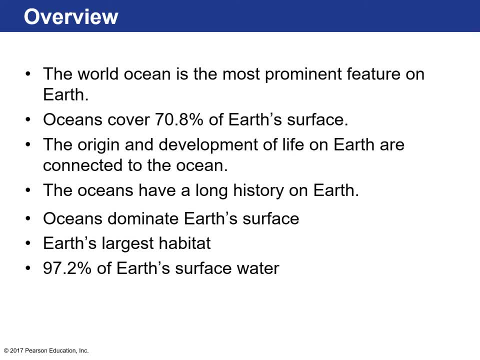 outer space you'd be looking at kind of like this blue blueberry covered in oceans and clouds and land makes up a smaller portion of that And the origin of life itself on our planet developed in the oceans. We're very connected to the oceans, In fact our own. 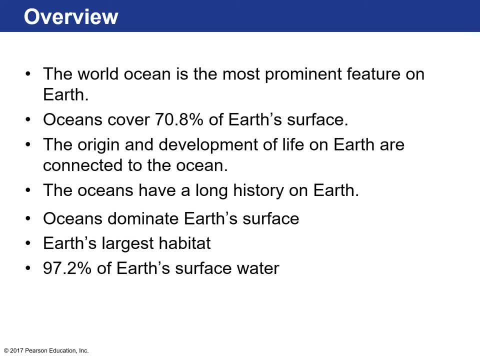 body chemistry is very similar to that of seawater, And the oceans have been around for billions of years. They have a long history on our Earth. They dominate the Earth's surface. It's the largest habitat. It contains the most largest number of living organisms. 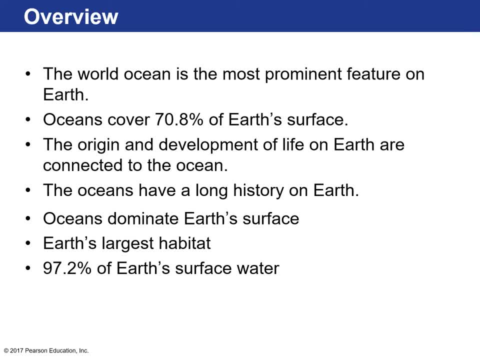 And 97.2% of the surface water that's found on Earth is ocean water. So the word Earth, or the way we refer to our own planet, is kind of a misnomer. We really should refer to it as oceanus or, I don't know, hydrosphere. 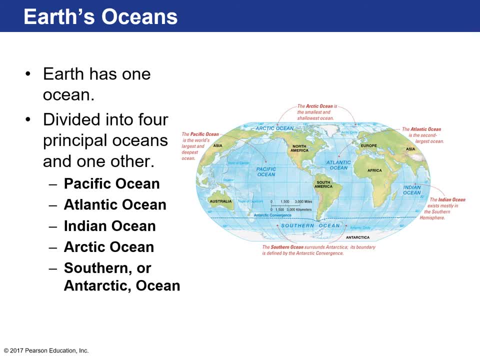 So let's talk about the different oceans. Now it really is one kind of one world ocean. All of these ocean basins are connected to one another, But we give them different names so that we know which area of the ocean you're referring to. So there's four principal oceans: The Pacific, 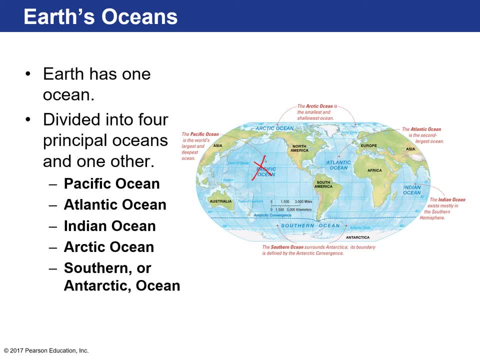 which you can find here. Okay, the Atlantic. Okay, we have the Indian Ocean And the much smaller Arctic Ocean up here. We do make a distinction right here. Anything just south of this latitude is referred to as the Southern Ocean or the Antarctic Ocean. 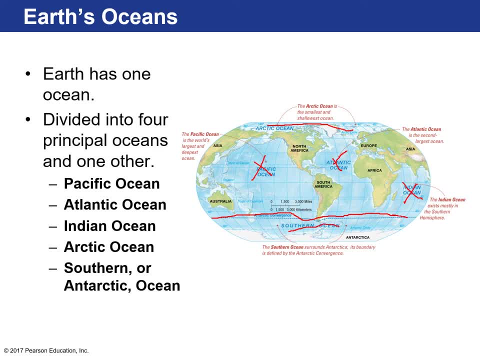 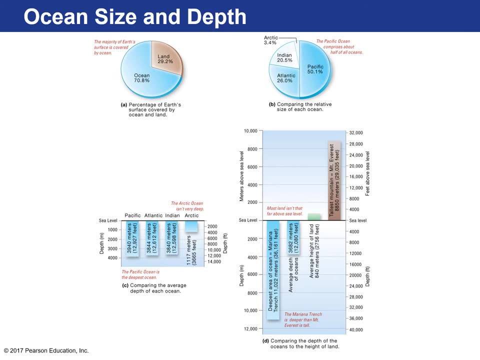 And the reason for this is because there's a major shift in global wind belts as well as ocean circulation that kind of splits these water masses or makes them distinct from one another. So here on the, on the top, you can see a pie chart of the coverage on Earth: 70% of the Earth's. 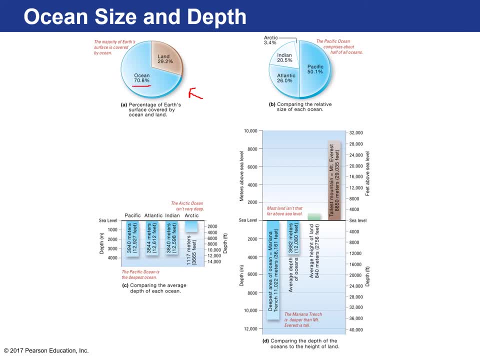 surface is the ocean, So if you just happen to be crash landing on Earth, you would probably hit water. Okay, only about 30% is land. Now if we break that down into the four different major oceans, the Pacific makes up about half of that. The Pacific is really big. 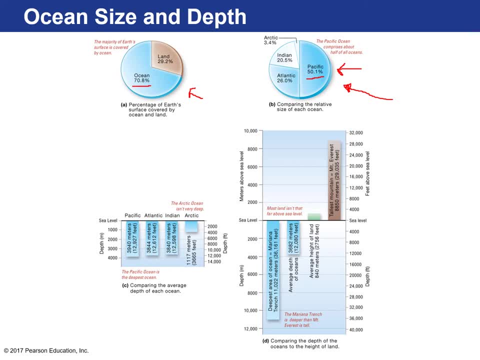 You can actually rearrange all the land masses and you could have them be kind of fit into the area that encompasses the Pacific. That's how big it is. That's how crazy it is like if someone gets lost at sea in the Pacific. 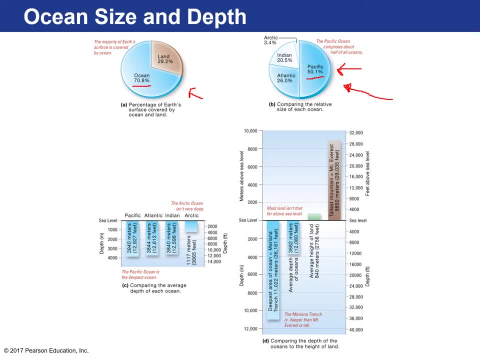 they might as well just kiss their lives goodbye, because they could be gone there for months. The Atlantic is about a quarter or half the size of the Pacific And the Indian Ocean is slightly smaller. The Arctic is really small over here, only maybe a quarter, maybe a bit smaller, Let's see. 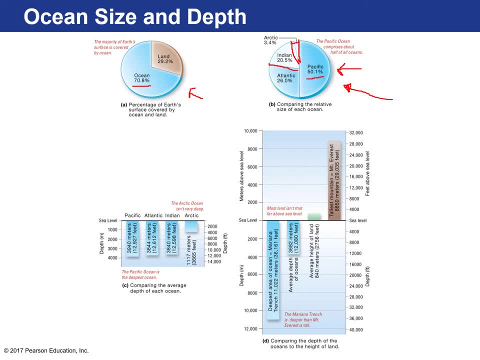 The Arctic is really small over here only makes about 3.4% of all ocean water. Okay, in terms of depth, this is depth here, So from sea level or the surface, where we would hang out, down to 4 kilometers here. 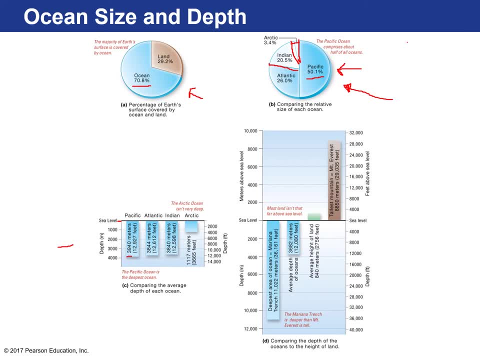 The average depth, Pacific is the largest and also, on average, the deepest ocean. Okay, Atlantic is not too far behind, just slightly shallower. as well as the Indian Ocean, The Arctic Ocean is very, very shallow in comparison to the other three major oceans. 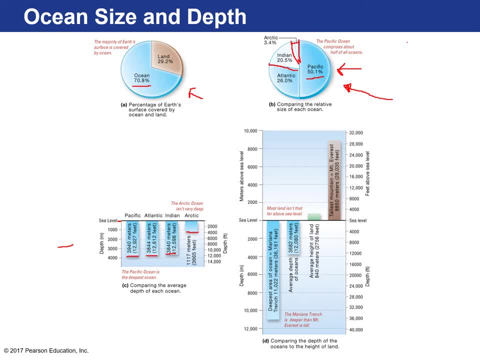 Now, if we compare elevation, okay, so this line right here designates sea level, So kind of like where we are in Florida. If you go kind of upwards on this y-axis, you're going up in elevation. Okay, so the tallest mountain on Earth is Mount Everest. 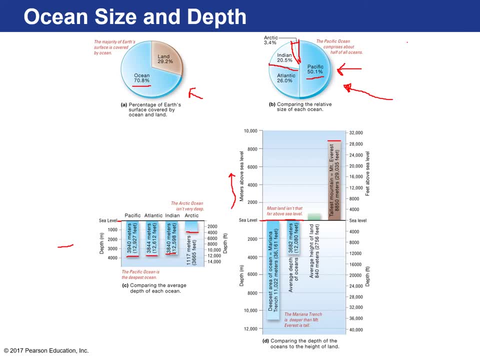 with an approximate elevation of about 28,000,. what is it? 29,000 feet, Yeah. 29,000 feet, Okay. so that's the highest you can get In elevation into our atmosphere on land. Okay, on average. the continents, however, are just kind of right here. 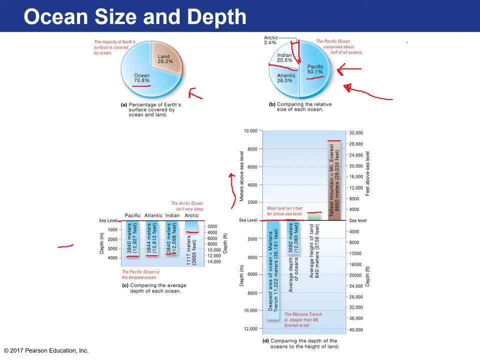 Okay, about 800 feet above sea level, And then, in comparison, this is the deepest part of the ocean, absolute deepest. This is the Marianas Trench in the Pacific Ocean, And that is 36,000 feet. Okay, so you could quote. unquote: 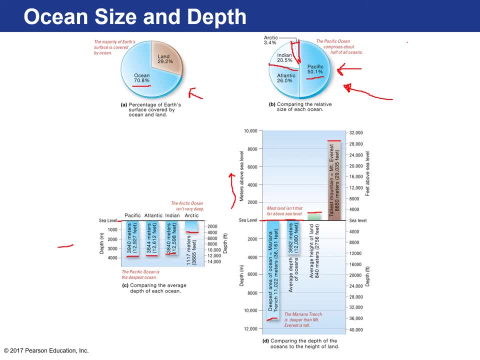 like: remove Mount Everest, drop it off the Marianas Islands in the Pacific, where the trench is, where the Marianas Trench is, and it'll fit, It'll completely submerge itself under the ocean. So that's how deep the Marianas Trench is, okay. 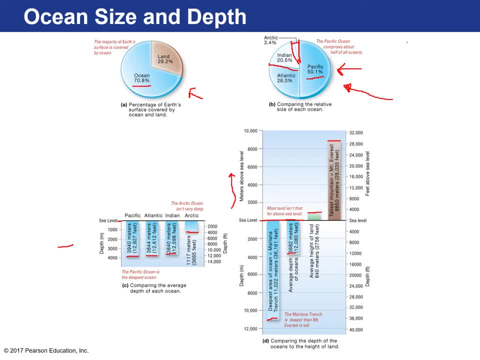 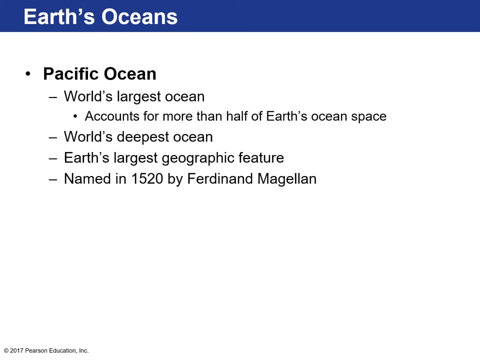 And then here is the average depth of all the ocean. So on average, if you were just to randomly drop somewhere in the ocean, you'd be almost about four kilometers below the sea surface. So that just gives you an idea of how vast and also how deep the ocean is. 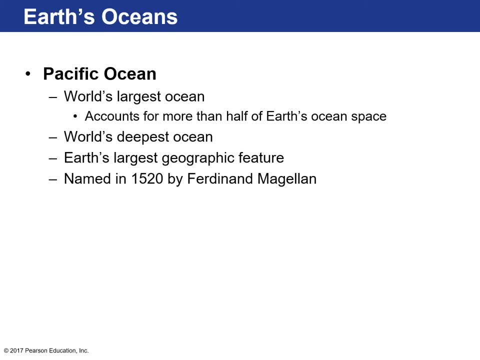 The Pacific is by far the largest, deepest And it was named by Ferdinand Magellan when he was navigating through the Pacific. He named it after its calm waters in 1520.. Okay, the Atlantic Ocean is about half the size, as I mentioned. 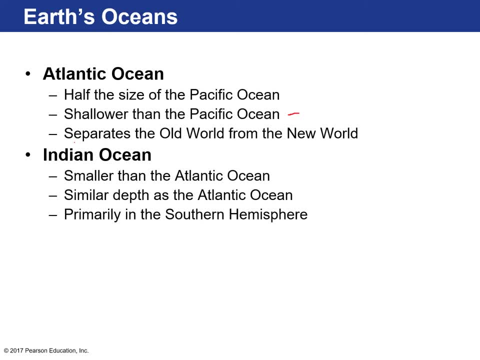 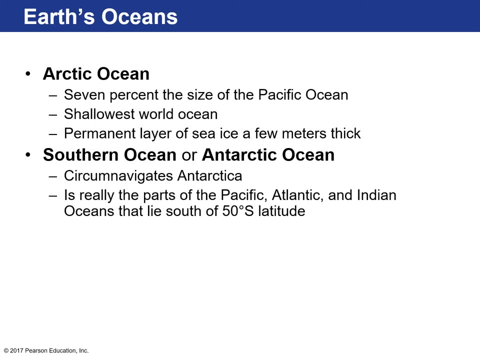 just a bit shallow. It separates the old world from the new. The Indian Ocean is much smaller, but it's as deep as the Atlantic and it's mostly in the southern hemisphere. The Arctic Ocean is a very small percentage in comparison to the other three major oceans, so it's also very shallow. 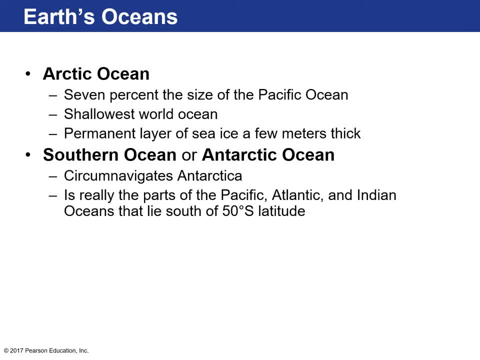 There also exists a permanent layer of sea ice that's a few meters thick, that sits on top of much of the Arctic Ocean. so that's a layer of ice that sits on top of the Arctic Ocean. And then there's that designation I mentioned before: the Southern Ocean. 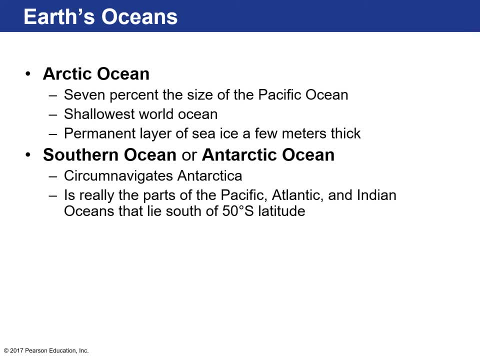 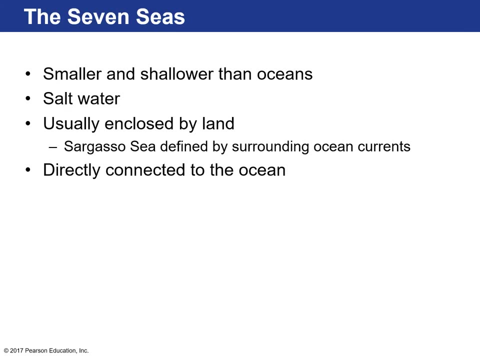 That completely circumnavigates the continent of Antarctica and it's essentially just parts of the Atlantic, Pacific and Indian, And that line of latitude, where that distinction is, is about 50 degrees south. Then there are the seven seas. I'm sure you've heard of them. 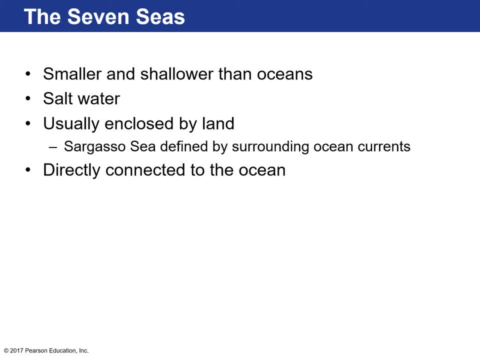 I'm sure you've heard of them, I'm sure you've heard about the seven seas in, perhaps, movies or books, or quoted in songs or something like that, But these are large bodies of water that are much smaller than the ocean and they're much shallower. 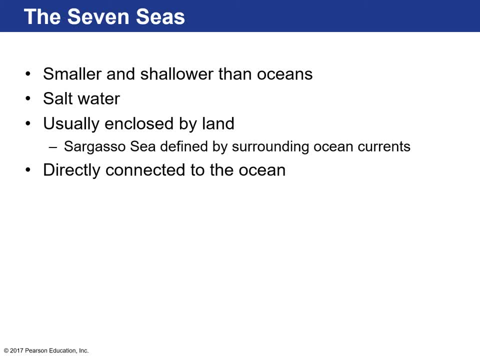 They all have salt water, but they're usually very enclosed by land but with at least kind of like a direct connection to the ocean. It's not always the case. One kind of exception is the Sargasso Sea, which is it's just east of the United States' eastern seaboard. 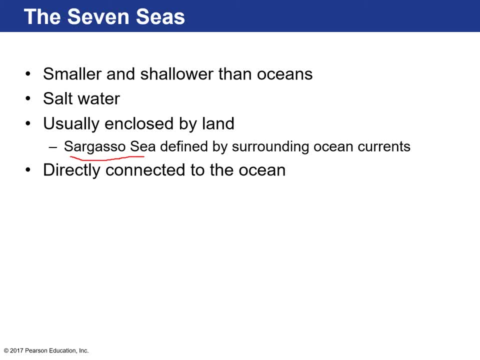 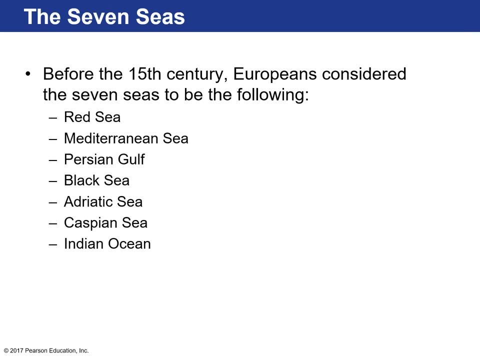 And it's given that name because of the sargassum, or algae that is often caught floating around the surface there. So yeah, these are the seven seas. Before the 15th century, the Europeans considered these to be the seven seas, the Red Sea. 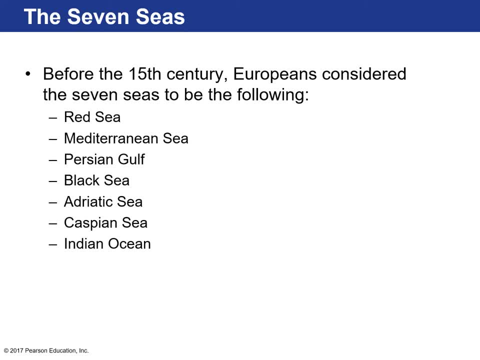 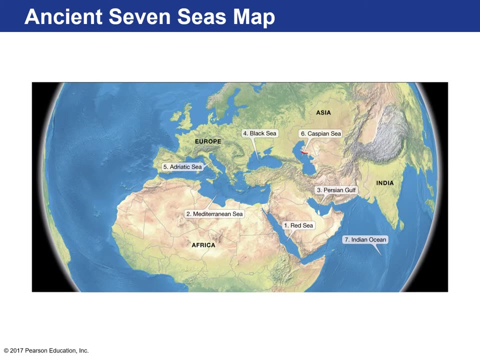 which is in the middle of the Atlantic, In between the African continent and the Arabian Peninsula, the Persian Gulf, the Black Sea, Adriatic Sea, Caspian and Indian Ocean. So here we can see, here's the. the Caspian Sea is actually a lake because 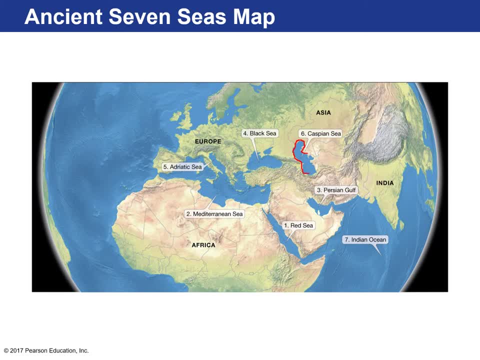 but since there's the evaporation rates are so high and there's so much input erosion from the local land area, it makes it really salty. Here's the Black Sea. Here's the Black Sea, Here's the Mediterranean Sea, the Adriatic Sea, right here Red Sea. 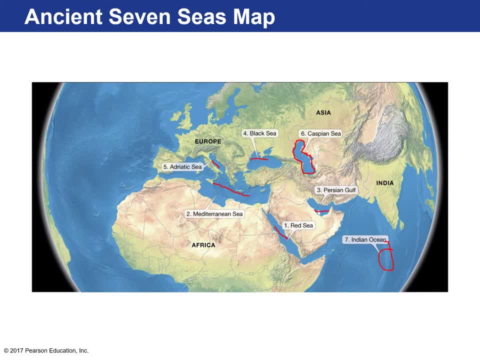 the Indian Ocean and the Persian Gulf. And so the reason historically, the reason why these are named the seven seas, is that this is largely where civilizations existed that had written history and navigated the oceans, And so they kind of traveled in these areas and that's why they had the 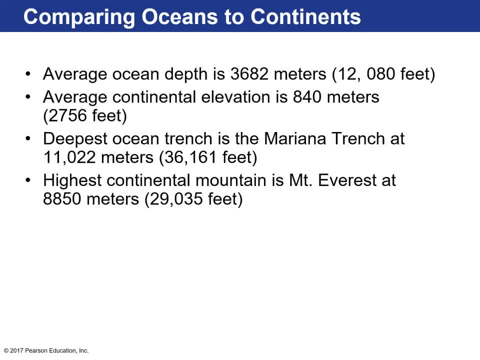 they named them the ancient seven seas. So the average ocean depth is 3,600 kilometers, which is about 12,000 feet. The average continental elevation places where we live is about 840 meters. excuse me, I said feet before, but it's actually meters. 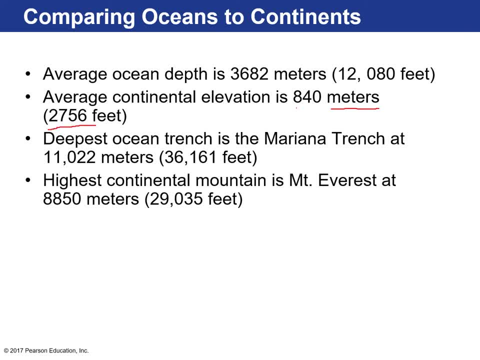 It makes it much higher, almost three times higher. That would be 2,756 feet. The Marianas Trench, the deepest part of the ocean, is about 36,000 feet. Again, to put that into perspective, the ocean is about 840 feet. 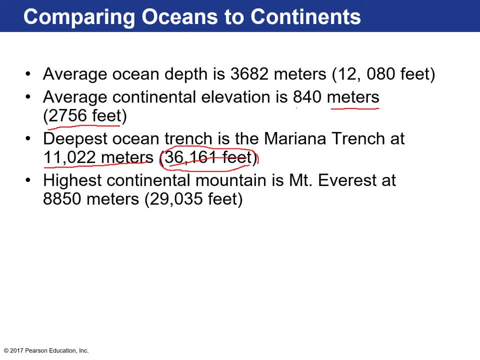 So to put that into perspective, what this means, if you've ever been on an airplane, or if we'll ever go on an airplane ride again, right, but when you're at your cruising altitude- typically that's between 30 and 35,000 feet- 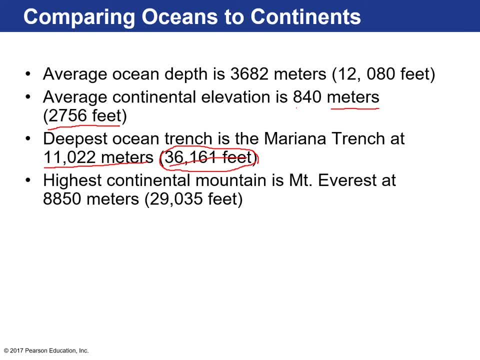 So imagine that. So imagine where you're sitting up there just munching on some peanuts, that giant bag of peanuts. they give you all three of them. you're chewing on that. The distance from you sitting on that airplane, traveling 400 miles an hour in an aluminum can. 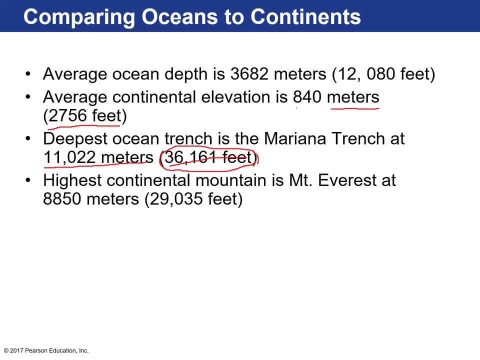 towards that. distance from there to the surface of the Earth is the same distance from sea level all the way down to the bottom of the Marianas Trench, And that distance is larger than the tallest mountain on Earth, Mount Everest, which is 29,000 feet. 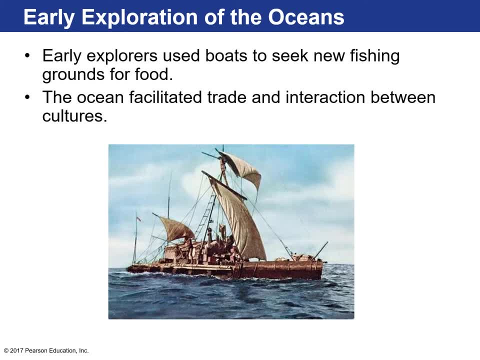 All right, so let's talk about some of the early explorers of the oceans. The oceans are really tied to a lot of human history, A lot of civilization. A lot of civilizations settled near the oceans for a bunch of reasons. Number one: food right. 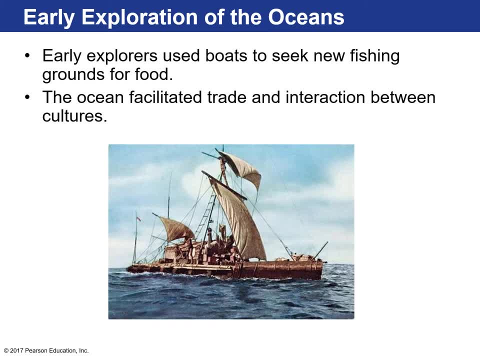 You know the ocean provides a lot of really tasty, high in calories, high in nutrient food, oysters, fish, you know, lobsters, whale, blubber, stuff like that. It also is very advantageous for trade and movement, right. 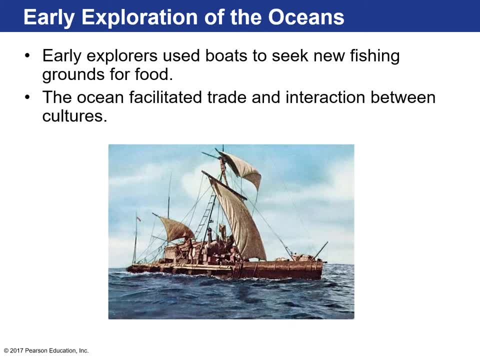 Once people figured out that they could build vessels and take advantage of current currents and wind patterns, all of a sudden you didn't have to walk all the way to go check out your friends in a different town. You could just drift or let the current take you or the wind blow you right. 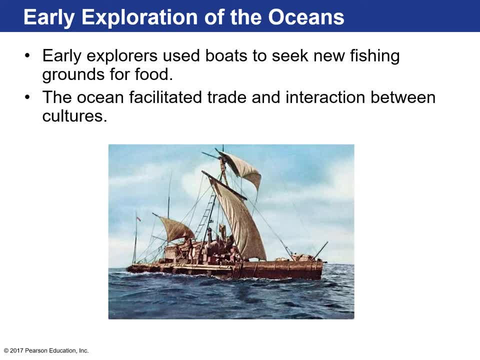 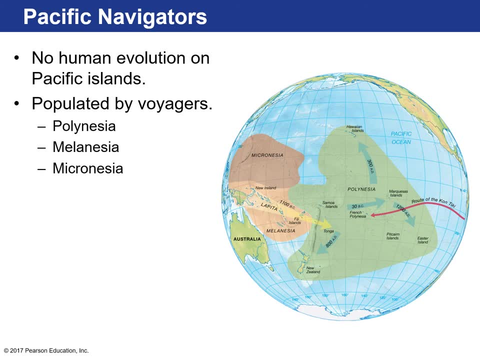 So, yeah, the ocean really facilitated a lot of trade and interaction between the cultures. That's why that was very prominent early on in human history. Some of the best navigators and the earliest navigators really were the Pacific navigators. Now, If we look at today from genetic studies, if we look at all the different islands leading 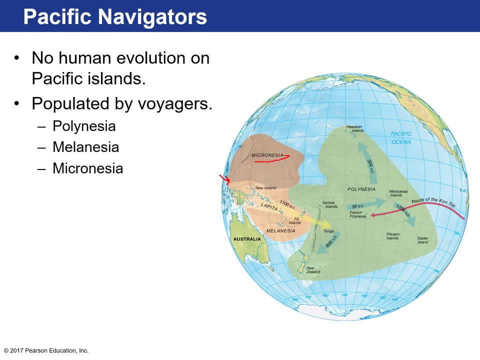 off from Southeast Asia and into Micronesia. here's the Marianas Trench. by the way, Guam and the Marianas Islands are over here, including Melanesia, all the islands here, New Zealand included Fiji, and here's Australia and then going into, or here's, New Zealand. sorry, 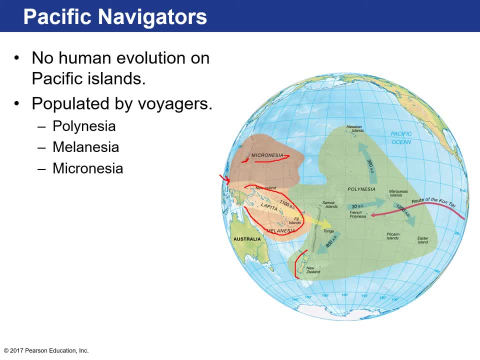 and into Polynesia. Genetically these people are very similar and they didn't evolve on their own, isolated from other peoples. What that means is that the very first travelers from Southeast Asia. they basically made it to all of these different islands in the Pacific Ocean and basically island hopped and moved. 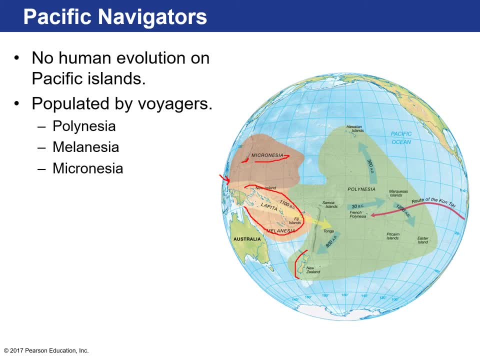 around. Okay, So these were voyagers, We were voyagers, Right, Yeah, So these voyagers were skilled, daring, they took chances and I'm sure a lot of them perished at sea looking for a new island to colonize. but obviously many were very successful because 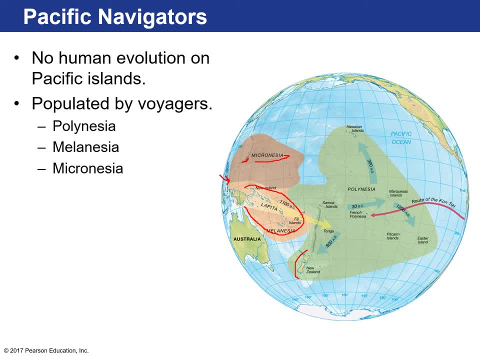 there are many different people and cultures inhabiting all of these islands that are here But based on archeological evidence. Okay, Here's the timing of their arrivals, Okay, And these change if there are new discoveries. but in Micronesia and a lot of the islands, 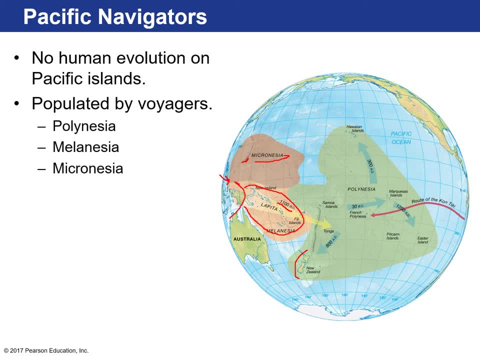 over here. there's evidence that there were humans here 4,000 years before the Common Era, Okay. And then going further and further away into towards Polynesia, then 1,000 years before the Common Era, Okay, 1,000 years before the Common Era is where we see Fiji, for example, colonized. 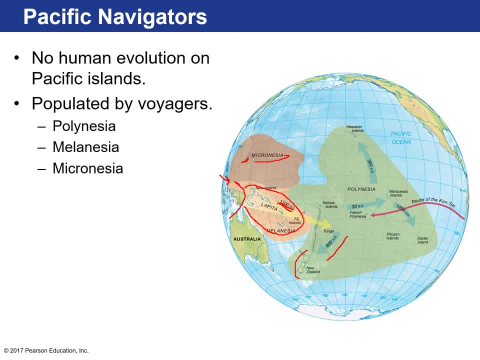 New Zealand down in this way: 800 after the Common Era. French Polynesia, 30 BCE. The Hawaiian Islands, about 300 years after the Common Era, Okay, And then Easter Island, about 1,200 AD. 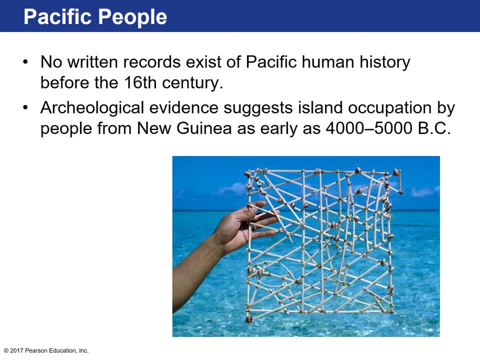 Okay, So there really isn't any written records of their history, so it's very difficult to piece together how they navigated this area, but they were incredible. Some of the things that they've discovered are these really cool maps, so to speak. 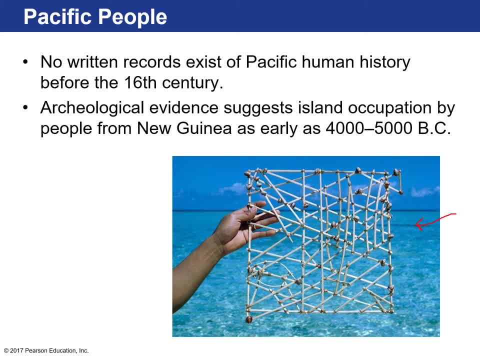 It's almost like an ocean guideline. It's a bunch of kind of palm twigs tied together And it might not look like much, but what it is is what it indicates to these navigators- are different patterns of open ocean waves. Okay, 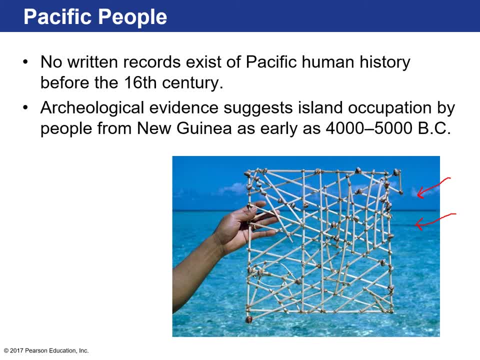 So these people were really in tune with the ocean. When they would go out and navigate, open ocean waves would approach and hit the ship right. For us land lovers, that would just make us sick: we'd be thrown up overboard. 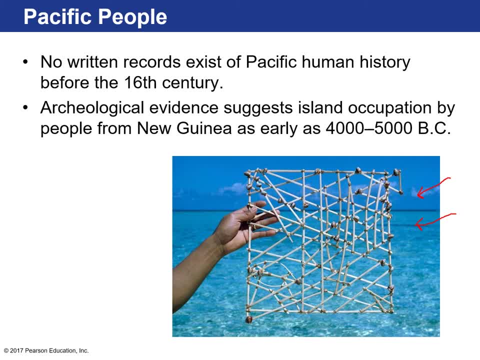 But to these people they could interpret the waves that were coming towards them. They could interpret the waves that were coming towards their boat And normally in the ocean you have open water waves kind of coming towards you and hitting your boat, But sometimes, as waves are kind of traveling through the open ocean, they'll interact. 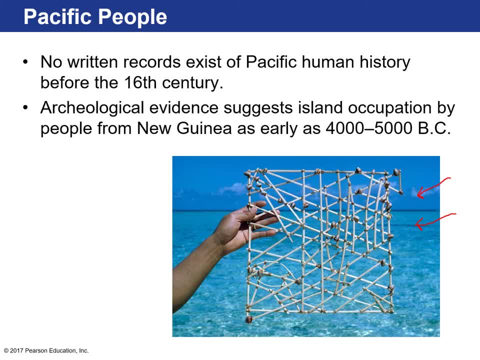 with land masses and they'll bounce off of them or they'll refract off of them, And that changes the pattern of the ocean- open ocean waves, And so what this guide, essentially told, indicated to these travelers was that they could navigate. 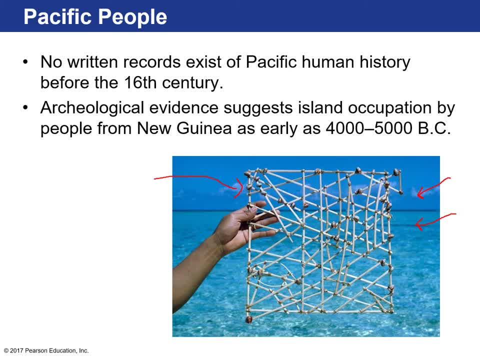 And so that's how they, our archeologists, think these pretty skillful navigators, interpreted the ocean to find new land. And so the idea is, a lot of these voyaging cultures maybe would inhabit an island and their population would grow. 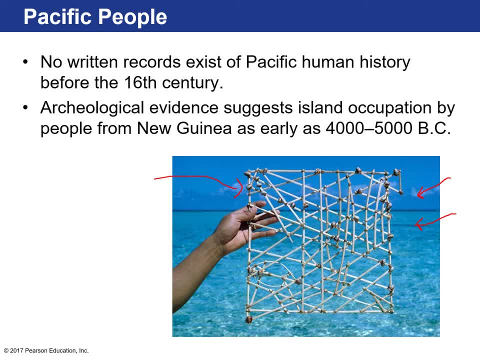 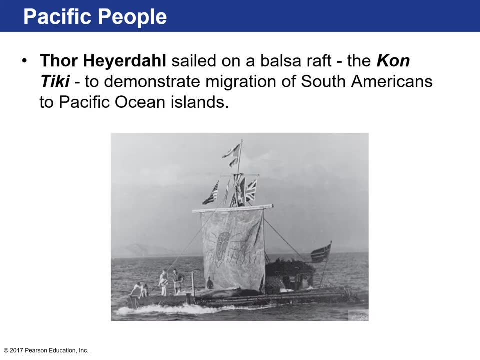 exceed the carrying capacity of the island that they lived on. so they're kind of forced to navigate and colonize somewhere new, and so that's why they'd send kind of like a group or settlement out to a new island. okay, so with new genetic studies scientists have kind of pinned down that all the, the, the. 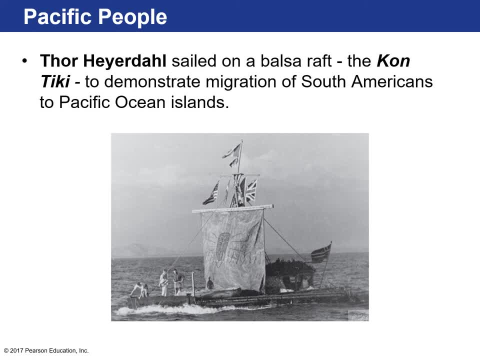 populations that have inhabited New Zealand, native populations that inhabit New Zealand, Australia, New Guinea, Fiji, Hawaii. they're all descendants genetically from people that originated in Southeast Asia, specifically areas near Taiwan, which is pretty cool and that was, you know, a big step in the research and understanding. but before that, there was this one researcher from: 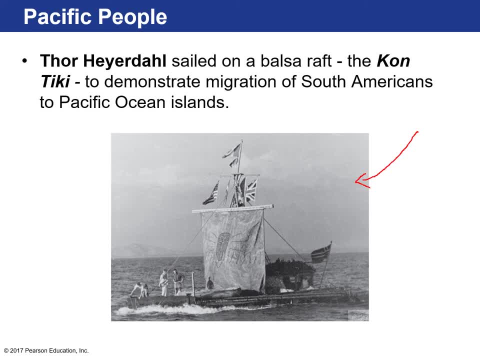 Norway, who was convinced that perhaps there were kind of two competing theories. one was the way people navigated to all these islands in the middle of the Pacific Ocean was through Southeast Asia, island hopping and navigating that way. but Thor Herondal suggested that perhaps some native cultures from South America made 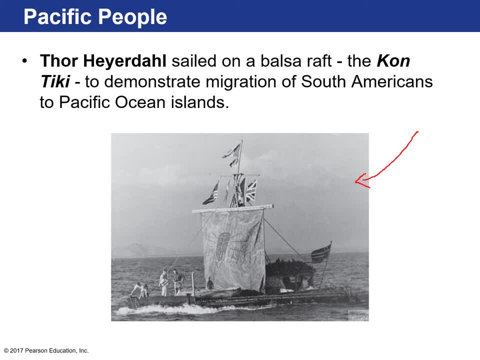 it to like Easter Island and then perhaps to Hawaii or something like that that was proposed. so he actually wanted to demonstrate that, so he built his own balsa raft, which you can see here, and he left from South America and made it to Easter Island, which was an amazing journey, but ultimately through genetics. 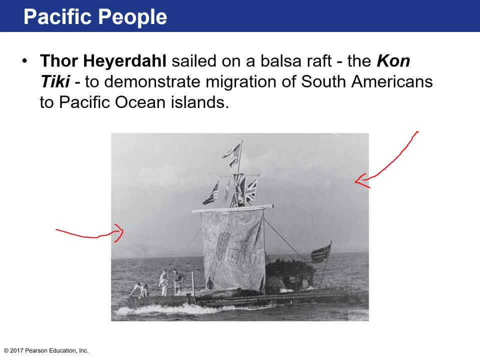 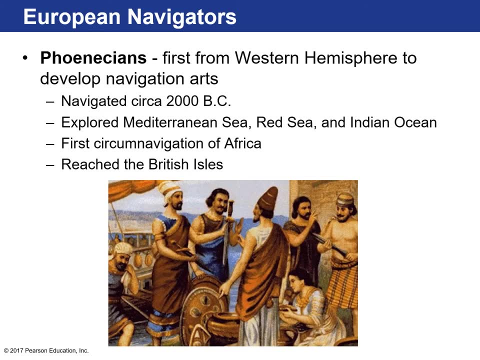 they kind of proved that the, the native people from South America, aren't related to the Polynesians. okay, so let's jump over to the European continent and the European navigators, much later, closer to 2,000 years before the Common Era. but the Phoenicians were credited with, kind of like, being the first explorers in in. 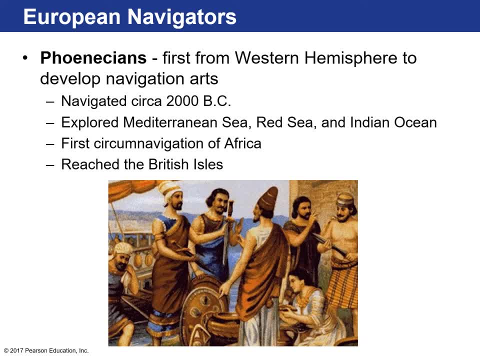 Europe, the first in the Western Hemisphere, I mean- and they get the credit because we have written history and evidence of it- and they explored the Mediterranean Sea, the Red Sea, the Indian Ocean. they were the first to circumnavigate Africa and they even reached the Mediterranean Sea in the 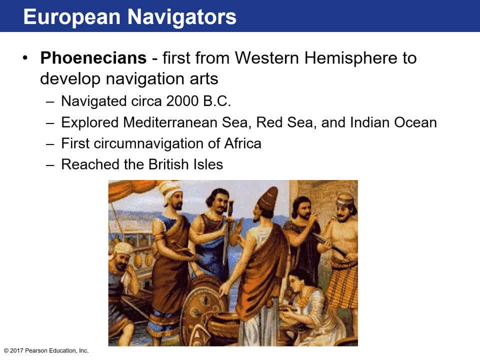 British Isles. the Phoenicians also developed our alphabet right, and the reason why that's important is because in order to kind of trade with different cultures, you kind of have to develop a system where you can, you know, trade on or communicate on even terms, and so developing a language and writing stuff. 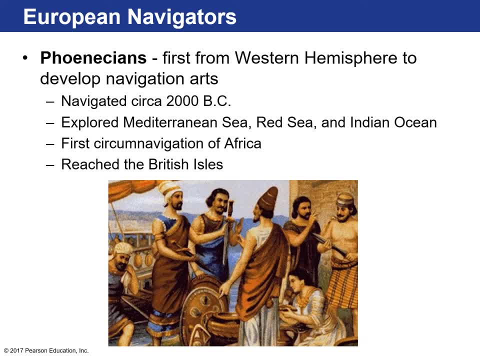 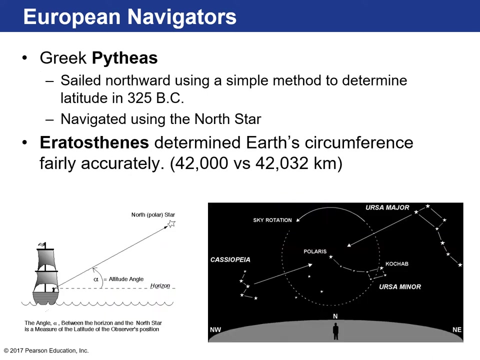 down was really important. so there's a lot of written history of travels, ships, logs and and materials like that and that those were the Phoenicians and the Phoenicians are found in like kind of present-day Egypt, Jordan, Israel, that kind of region. okay, the Greeks kind of came afterwards and with the, the Greek 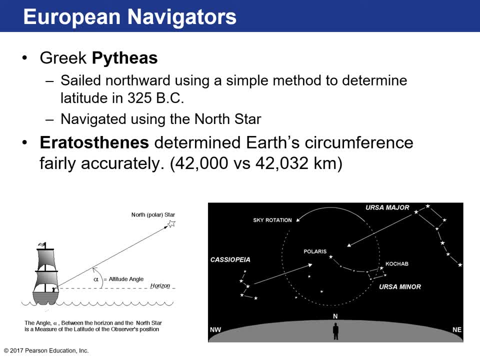 civilization. there was a huge rise in scientific thought and great kind of institutions were being built, like the like the library of Alexandria, and there was a lot of progress in terms of scientific progress. and they used these technologies in their sailing. and the Greeks sailed northward using a very simple way to determine the, the latitude. 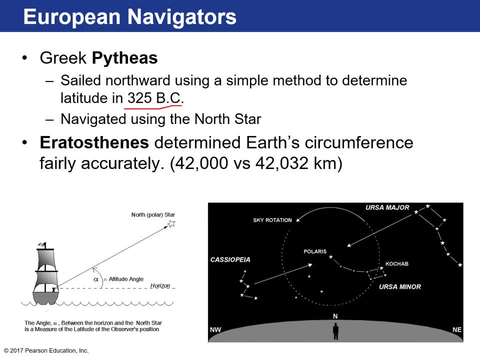 that you're at meaning like how far north or south you were on our globe to okay, and the way you do that is by using the North Star. so wherever you are, let's say you're here. the North Star is approximately kind of like on our axis. 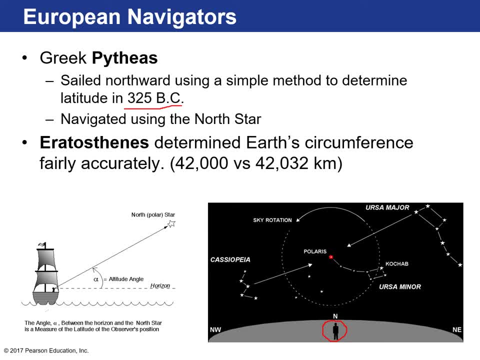 that goes right through our, the sphere of our Earth, and so if you're at a more northern latitude or closer to the kind of the northern or the North Pole, Polaris will will be higher up into the sky. if you're closer to the equator, Polaris will be seen closer to the horizon, and so that angle, right that's. 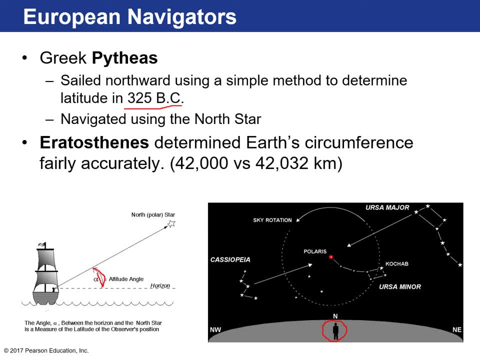 this angle. here you can measure that. if you're on a boat, you can measure the angle difference between the horizon and the location of Polaris. so if Polaris is higher up in the sky, that means you're at a hot, more northern latitude. if Polaris is down here, at a really, really just above the horizon, that means you're. 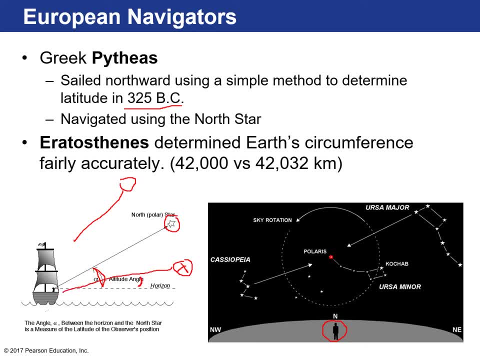 pretty close to the equator so you can determine your latitude based on that angle? okay, but you couldn't. at that time they didn't know how to determine longitude, meaning your east-west. that was developed much later, later and back then. okay, this is 300 years before the Common Era. the Greeks knew the earth was. 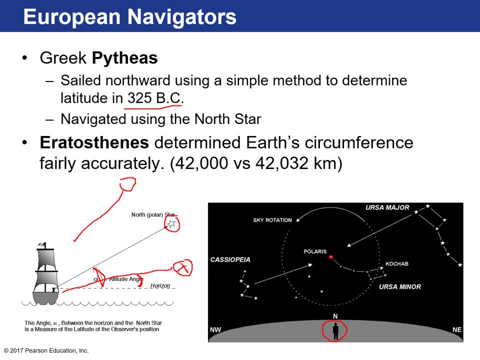 round, okay, and it was determined by Eratosthenes. he basically used simple geometry and he compared how a stick cast a shadow in one town versus another town, which a known distance away from that stick, and the at the same time the Sun kind of directly shown through directly above a well, and he used that. 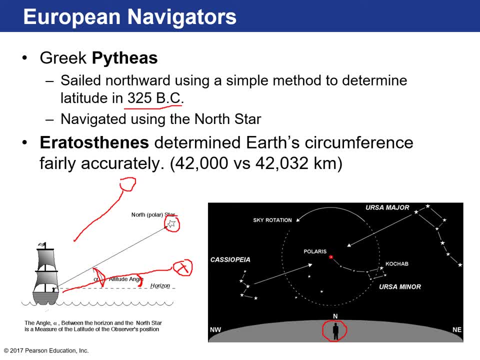 to calculate the circumference of the earth, he came up with a number: 42,000 kilometers, right 300 years before the Common Era, and the true number of the circumference of our earth is 42,000, 32 kilometers, and that is remarkable that he was able to calculate with that level of accuracy 300 years before our Common. 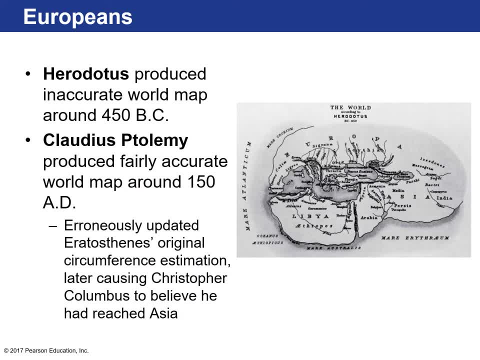 Era, which is, which is pretty incredible. later on there were other Greek scientists who updated erroneously here Eratosthenes circumference measurements, but they, what they did do was provide the most accurate a quote-unquote world map. right, because this was their world at the time. they couldn't really explore. 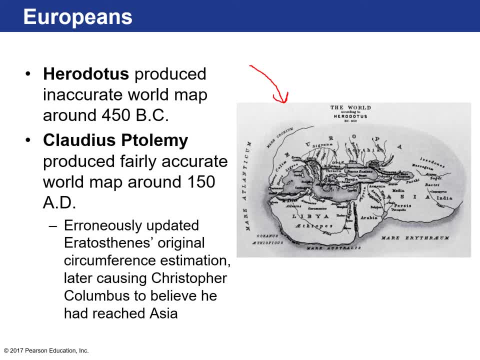 much farther than this, but they were able to draw longitude and latitude lines was just pretty impressive for that time. okay, this was in 150 AD, so I vollum e updated the circumference estimation and that became. you know, that was used by Christopher Columbus as he believed the earth was. 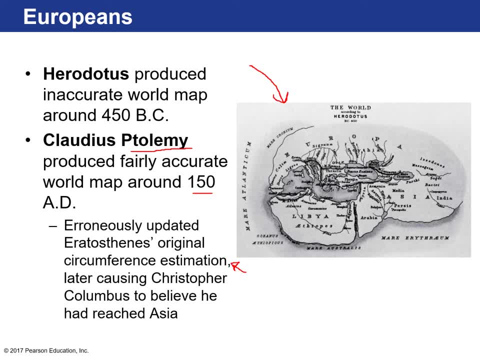 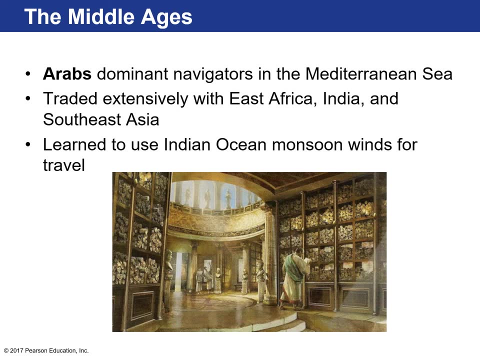 much smaller than it was because of this erroneous at calculation, and that's why he thought he can make it to Asia, axis, saling, West in the Atlantic, and then, And so the Middle Ages came about, and there was a big tragedy: The Library of Alexandria burned down because there was a rise in the beginnings of Christianity. 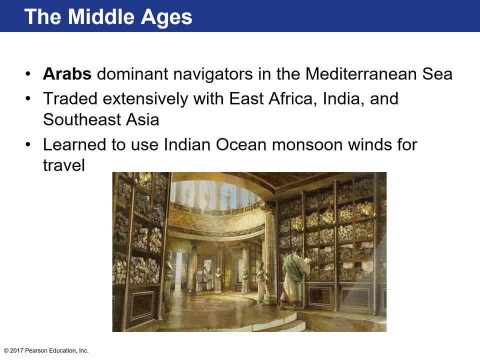 and they kind of took down the Roman civilization, burned down the Library of Alexandria where all these ship logs and poetry and literature and mathematic documentation was stored, and so all of that precious information was lost and the Western Hemisphere kind of dipped into the Dark Ages. 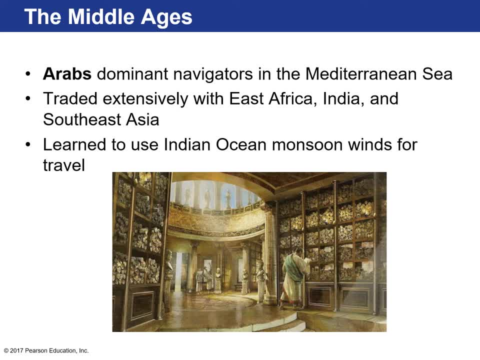 But there were a few Arab scholars that actually copied a lot of the information from the Library of Alexandria and they took that with them and then they became and used that knowledge and became the dominant navigators in the Mediterranean Sea, And so they traded with East Africa, India and Southeast Asia predominantly, and they 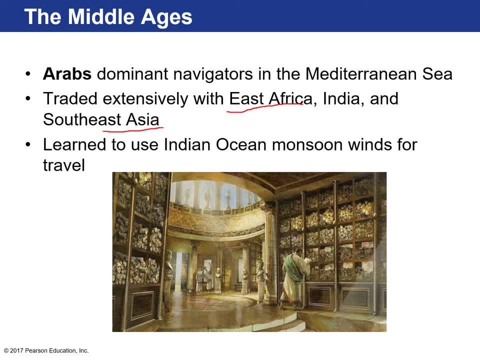 took advantage of the monsoon season, And so when the monsoon winds come in, they go into India, they dock there for a while, bring in materials and trade things that they want, buy some other things that they know at home that they would want to buy, and then, when the winds shift, they would go back home. 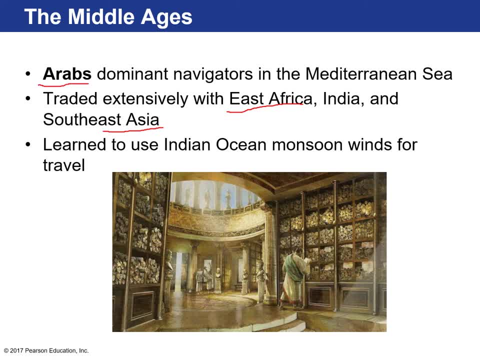 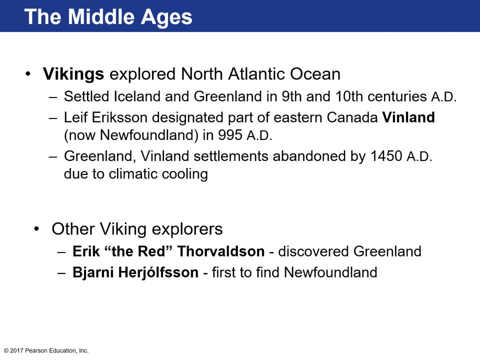 So Arabs during that time became the dominant navigators in that region. In a different kind of completely different era In Northern Europe the Vikings explored Iceland and Greenland in the 9th and 10th centuries AD. Leif Erikson looked at, made it down to Canada and Vinland, which is now known as Newfoundland. 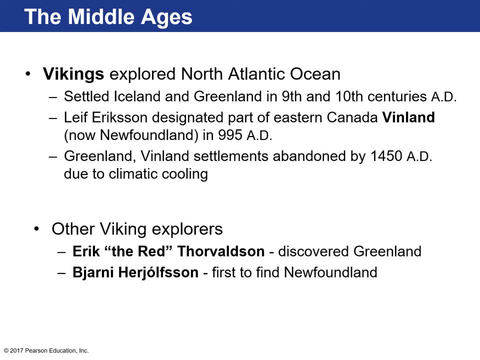 by 995 AD. There were actual settlements in Greenland and in Newfoundland in 1450 AD. So the Vikings explored Iceland and Greenland in the 9th and 10th centuries AD. Leif Erikson looked at, made it down to Canada and Vinland, which is now known as Newfoundland. 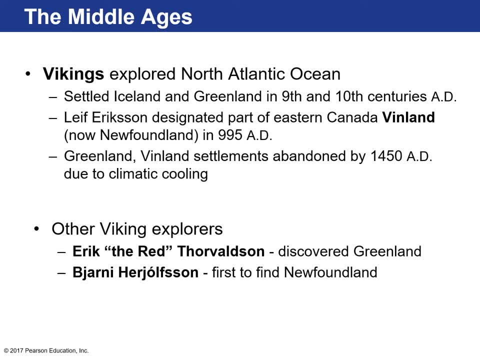 by 995 AD. The Vikings explored Iceland and Greenland in the 9th and 10th centuries AD. The Vikings explored Iceland and Greenland in the 9th and 10th centuries AD. People are Viking explorers after Leif Erikson. like I'm going to butcher this name, but 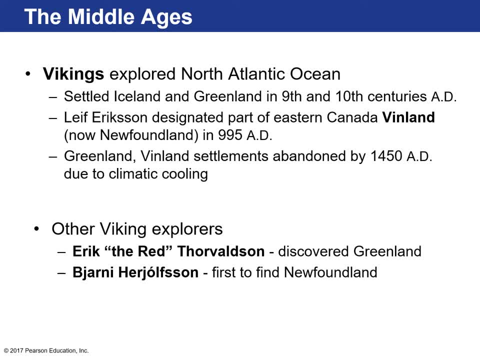 Bjarne Herjolfsson. they actually developed settlements But the problem was they had some pretty bad weather some of those years. there were some pretty bad winters and their bad farming practices and those settlements kind of died out. But the Vikings are actually credited with that. 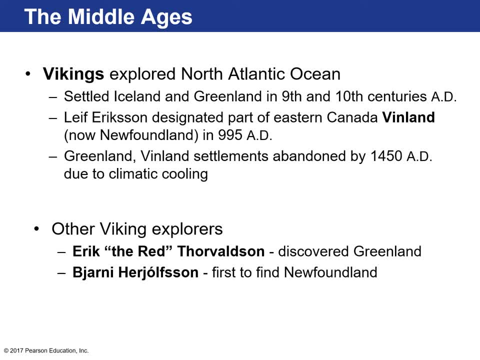 The Vikings are actually credited with the first kind of European cultures to settle in the Americas. Not actual, you know, not really Christopher Columbus, but the Vikings were actually there first, So they were pretty good explorers. They don't get. they don't get the credit I guess that they deserve. 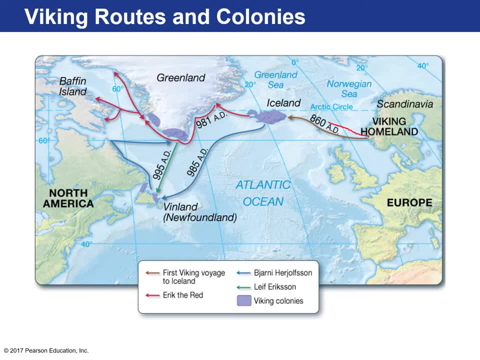 But here is, here is the Viking homeland. made it to Iceland, Greenland. Here are some few settlements over here. They think they explored areas into Baffin Island in Canada. And then here are those settlements in Newfoundland. Okay, but those largely weren't successful. 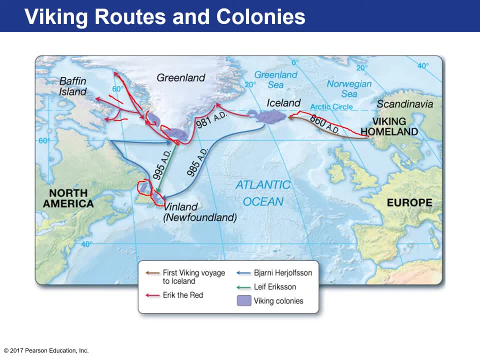 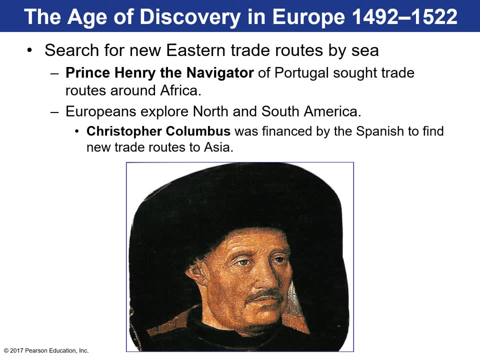 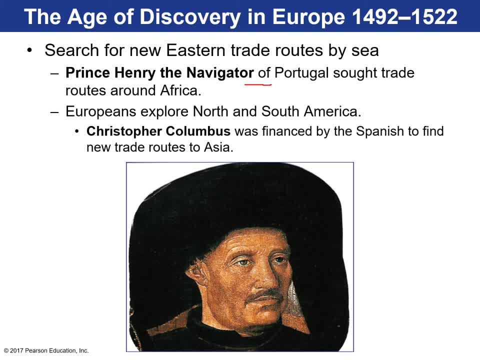 Okay, and then Europe came back into the picture. There's the Age of Discovery: 30 years from 1492 to 1522.. and under him other explorers kind of trained under him, like Christopher Columbus, and they were set to explore kind of different trade routes the most. 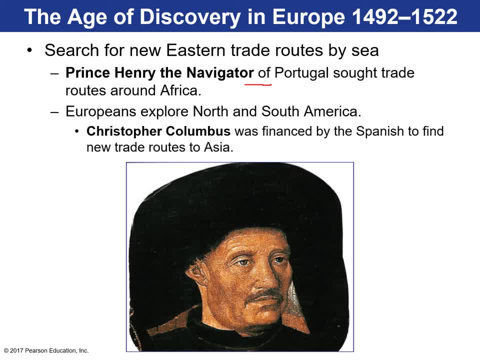 common one was to kind of circumnavigate Africa and go that way, but that was a pretty long and dangerous journey, and so that's why Christopher Columbus was able to finance a shot in the dark kind of route, and the Portuguese actually didn't finance it, but he was able to talk to the Queen of Spain and they financed his. 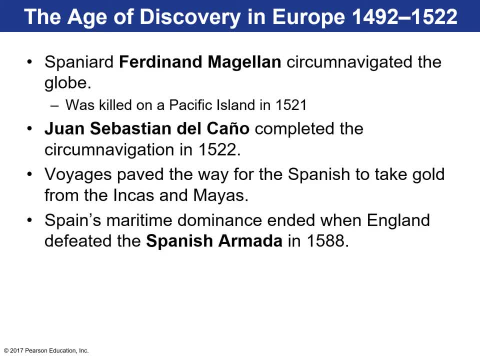 trip, and so he went out and landed in Hispaniola, which is present-day kind of Dominican Republic and Haiti, and he kind of found that and committed atrocities. he did some pretty bad stuff and kind of made a few journeys back and forth about three times, but he actually 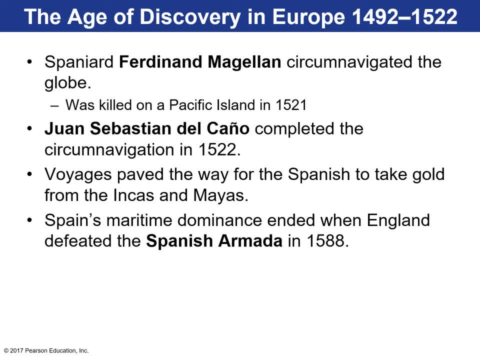 never set foot in North America, he kind of only set foot in the Caribbean. okay, then later Ferdinand Magellan was the first to undertake the circumnavigation of the entire globe. okay, there were. he went on a group of three ships and 280 sailors and he was able to do that, and he was able to do that, and he was able to do that. 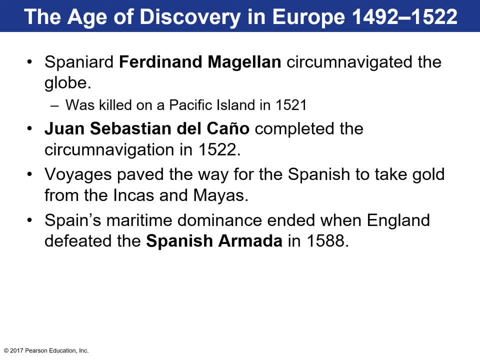 and it took him, I think, three years, three years out in the ocean, and he was killed in the Pacific Island in 1521, and one ship made it back to Spain and it had 18 sailors. so what are the odds of surviving that journey? pretty bad right. 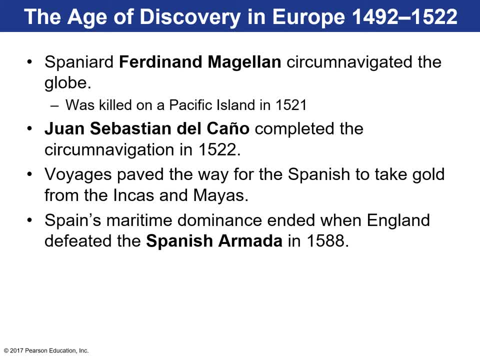 then Juan Sebastian de Caño completed the circumnavigation in 1522. okay, and those voyages really paved the way for the Spanish to kind of rule the seas at this time, and they just absolutely exploited the new cultures that they found in the Americas, in the Caribbean. 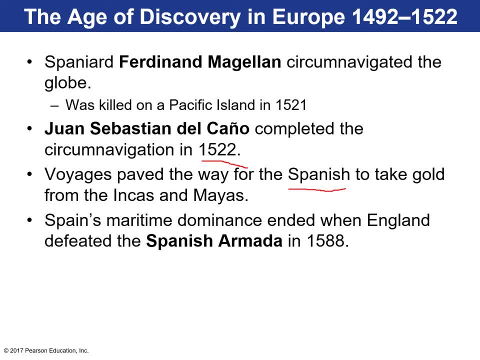 they essentially just took all the gold and silver as possible to go feed the greedy- you know- monarchs that they were serving right, and so they committed atrocities, and in Central America and in South America, and so their, their dominance in the Caribbean was basically during this time ended when English and also Dutch ships, which were smaller and also more 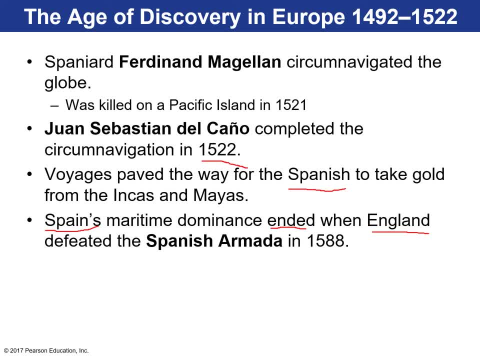 maneuverable compared to the giant Spanish galleons. So what the English and Dutch essentially did were like: oh okay, we'll just rob your ships and they'll take all the gold that they took from people in the Americas. And so they defeated the Spanish Armada by 1588.. And then 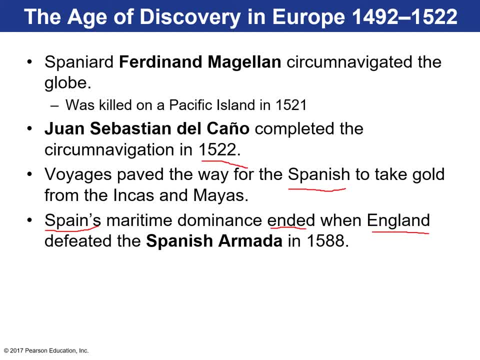 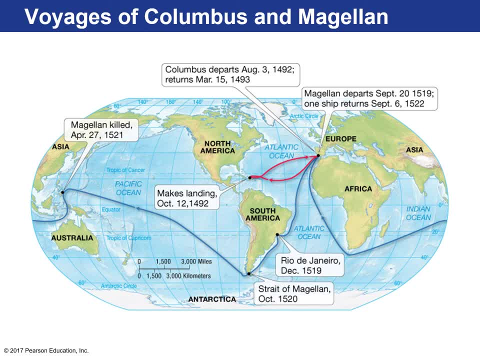 England essentially became the world colonial powers at the time when they defeated the Spanish Armada. Okay, so here are the voyages of Columbus. See, Columbus just kind of went down, made a stop and came back. He did that, I think, three times. And then this is Magellan's. 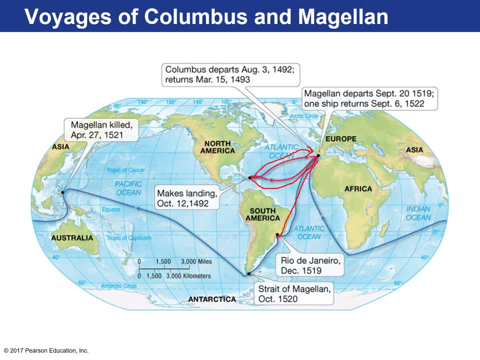 trip. So he went to Rio, right Straits of Magellan named after him, and then went to the Pacific Islands. He was killed here And then his crew kind of did the last little leg of the trip and circumnavigated the globe, which was a big deal, All right. Took him three years to do it. 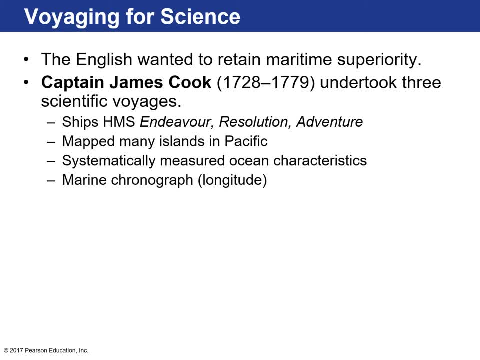 Imagine giving up three years of life just to do that. Probably dying, right, I mean odds are. I mean I would die, Most likely die. I get very seasick, Anyways. so the English: they wanted to retain their kind. 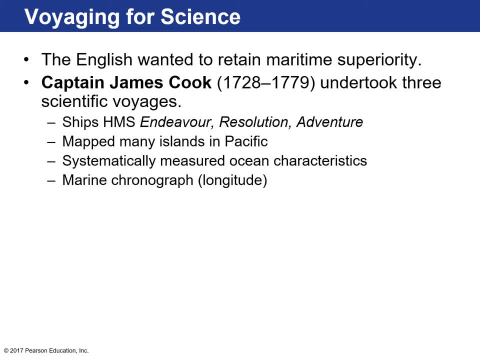 of maritime superiority And one of their best navigators was Captain James Cook, And the English were almost like the first navigators to go on voyages that were strictly for scientific purposes. So instead of just kind of going out and creating settlements and colonizing and exploiting different areas, 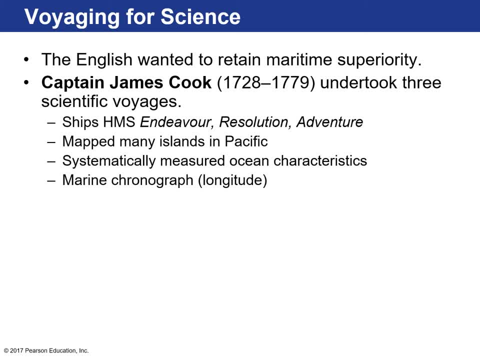 they actually sent out ships to find out new information, Things like finding perhaps pass through, like the Northwest Passage through Canada, find new islands. One of the trips James Cook took on was to go to Tahiti and watch Venus's trip to the Pacific. 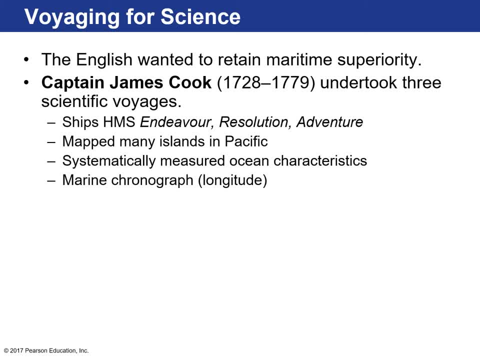 And he was able to track across the sun because they wanted to accurately measure Venus's orbit at the time. And he captained the HMS Endeavour, resolution and adventure And they measured a lot of ocean characteristics like sea surface temperature. They also did. 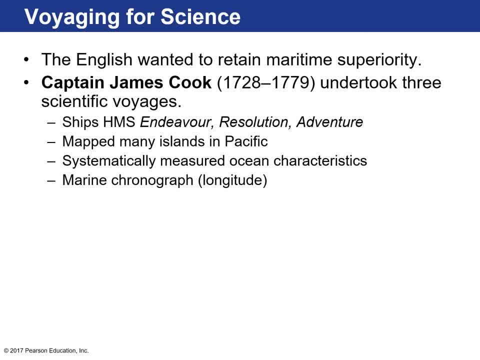 soundings, which are a measure of the depth of the ocean, which hadn't been done at the time, And they benefited greatly from new technology: the chronograph. This was developed by a cabinet maker in England. It's essentially a watch, And by being able to 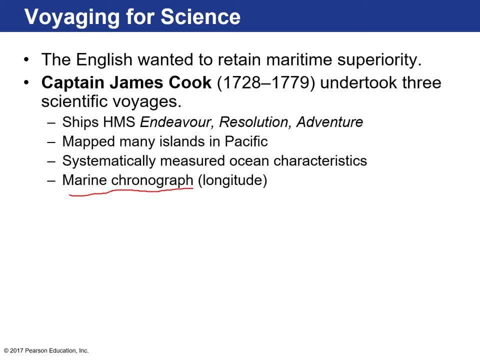 kind of tell time. independent of where you are, you can determine how far you are east and west and not just north and south. So that was a key development in being able to kind of pinpoint your spot or your location on Earth Using longitude and latitudes. In fact the English came up with that. 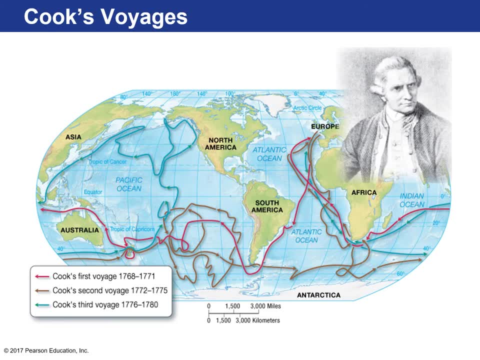 Okay, here were Cook's voyages, Kind of traveling a lot of different areas in the Pacific Ocean, And he was interesting You can read. he kept a really detailed journal, which is pretty crazy, because it's very interesting. You can read his journal. 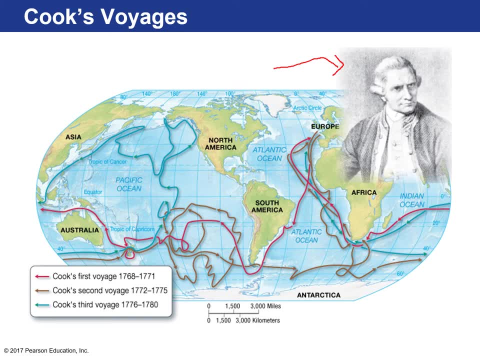 because he encountered people in the Pacific that had never met any other person ever. So it was kind of like the first person he met in the Pacific. So when he found out- or it was just a very sort of a shocking thing- that he encountered people in the Pacific that had never 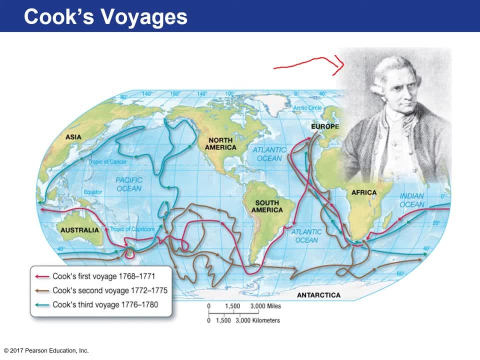 met any other person ever. So it was kind of like the first person that he met in the Pacific, So the first person encounter of, like you know. basically, these strange white people showed up out of nowhere in this giant wooden ship and then interacted with locals. so it's, it's. 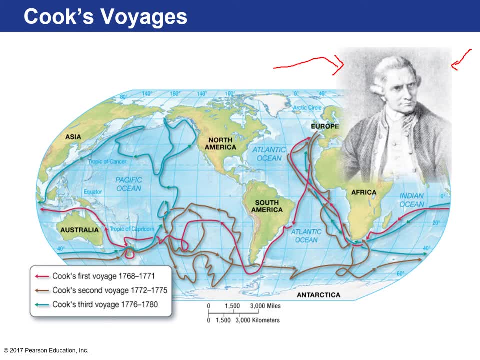 he has interesting insights and interactions with with native people. ultimately, he died in a skirmish with native people, most likely some sort of miscommunication or I don't know what happened, but he died as a result of skirmish in somewhere in the Pacific. he's also credited with a lot of sailors. 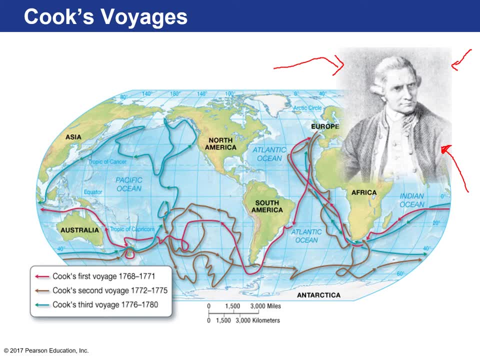 before the English kind of dominated the seas. at this time sailors suffered from scurvy right, and Pirates of the Caribbean really fantasizes what it was like being a pirate or being out in the ocean. but scurvy was a pretty big deal and actually killed more sailors than shipwrecks. 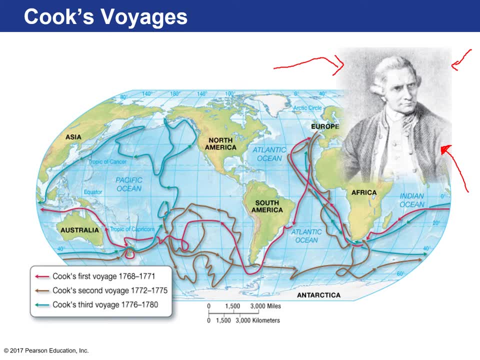 you know, encounters with natives and and and other perils that they are in the ocean and essentially what scurvy is is a deficiency in vitamin C. what happens is your teeth start turning black. immune system goes down. it's. it's pretty nasty being a sailor back then. was was horrible. so what he figured out was he? 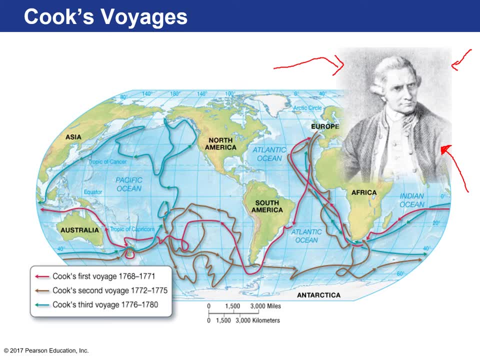 improved his sailors diets by introducing sauerkraut. I don't know if you ever had sauerkraut before. it's kind of like that. it's like a pickled cabbage, essentially, but that is loaded with vitamin C and it's also can be stored for a long time, so you can be on a ship. 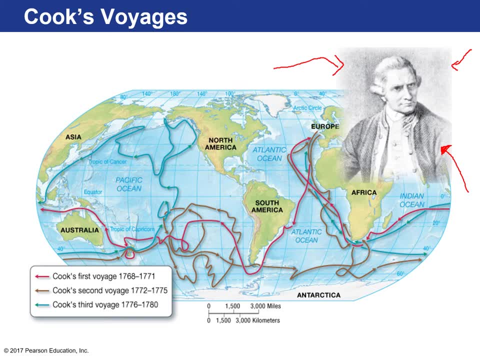 for two to three months and still be able to eat sauerkraut, and that actually improved the diet of his sailors and increased the rate of survival for sailors that went on these journeys. okay, so oceanography continues today and we'll talk about that later. 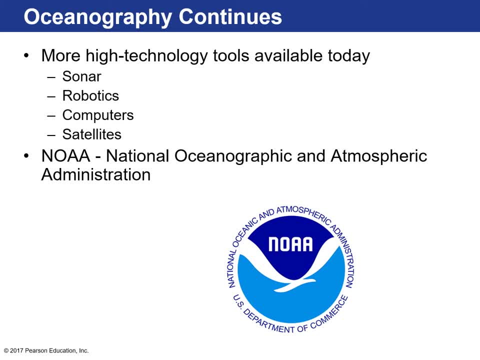 Thank you for watching. Obviously, today we have a lot better technology. We have sonar, robotics, satellites, computers, right. We have the National Oceanographic and Atmospheric Administration. That is a great agency that helps us predict ocean conditions and tracks hurricanes and stuff like that. 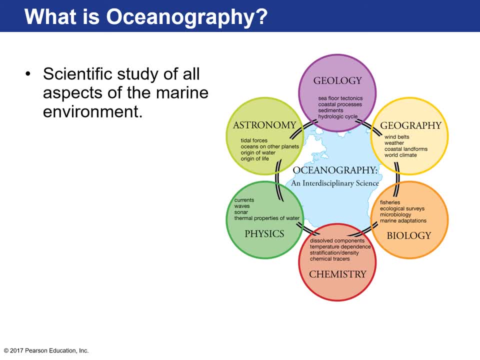 And so finally, here we are 30 minutes in And, yeah, you might be wondering what is oceanography? But oceanography is kind of like an interdisciplinary science that includes all kinds of different sciences together. In this class we're really just kind of we're going to skim the surface of a lot of different areas of science. 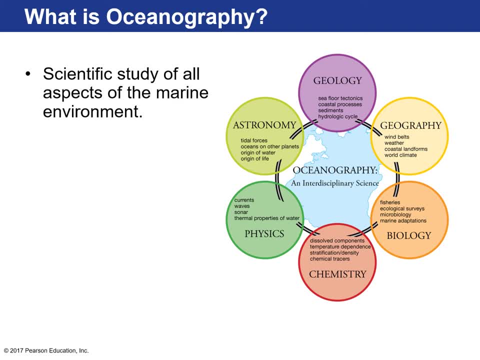 And I'm going to try to dive deep and get some meaningful context in a lot of these subjects. But it covers geology, okay: seafloor, tectonics, sediments, geography, wind belts, weather. Another science that's very important here is biology: fisheries. 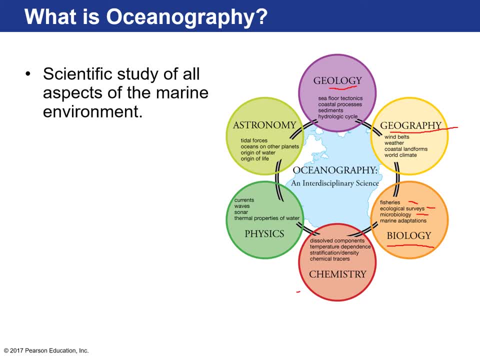 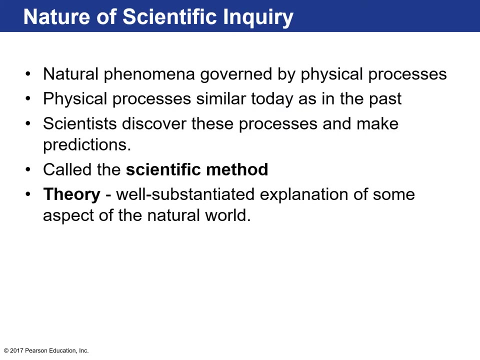 The ecology, microbiology, chemistry of the oceans, physics of the oceans, thermal properties of water, waves and currents, And then astronomy is important too, because that controls tidal forces and origins essentially, And so scientific inquiry is just essentially the phenomenon of trying to understand the physical processes on Earth. 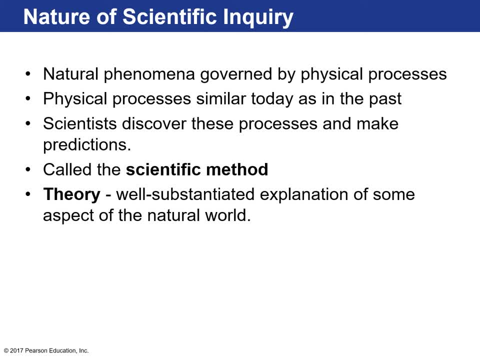 and being able to predict what will happen as a result of that, And so we're going to talk about that understanding. okay, The physical properties that we witness today, processes that we witness today, are similar than the ones that we've seen in the past. okay, 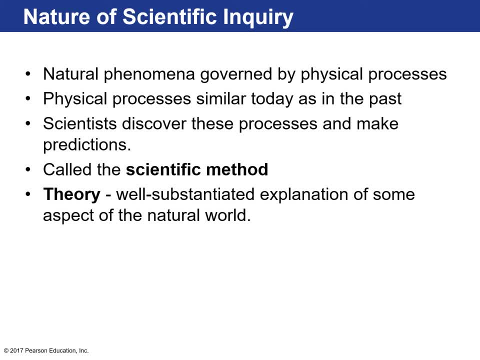 And so science tries to discover these and then make predictions, And we do this in kind of a logical method called the scientific method. And once observations and hypotheses have been made and then have been tested, and then vigorously tested, well, you come up with a theory. 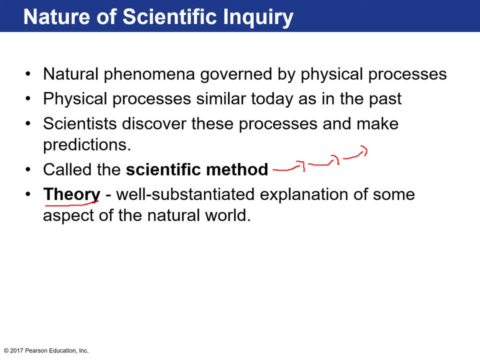 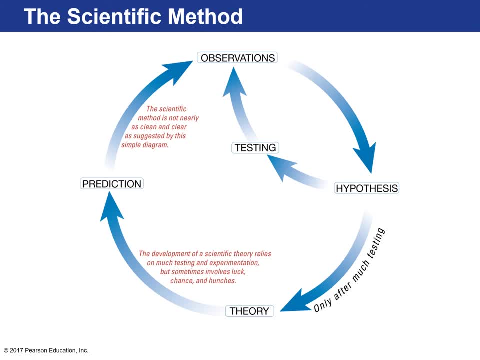 And the theory is a well-substantiated explanation of some sort of aspect in the natural world. okay, So here's that process. You start off with observation. The book does a pretty good job of an explanation. Let's like whales. 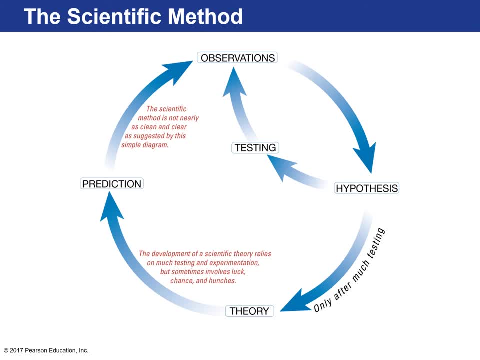 Have you ever seen that Prudential commercial where the humpback whale kind of jumps out of the water and breaches and then smacks itself back down? That's an observation right And scientists and regular people and sailors have always observed whales breaching in the water, kind of jumping out of the water and smacking back down. 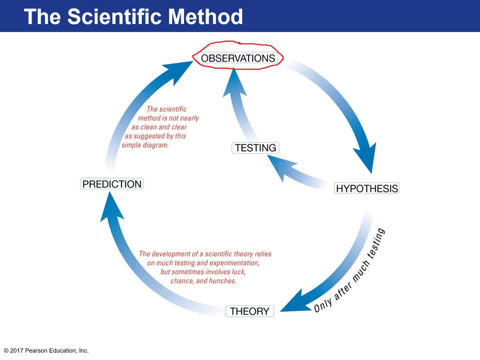 That's an observation, right. Why do they do that? That's an important question. Why do whales breach? And so you try to come up with explanations or hypotheses on why they do that. Do they breach because they're communicating with different pods of whales in really far distances? 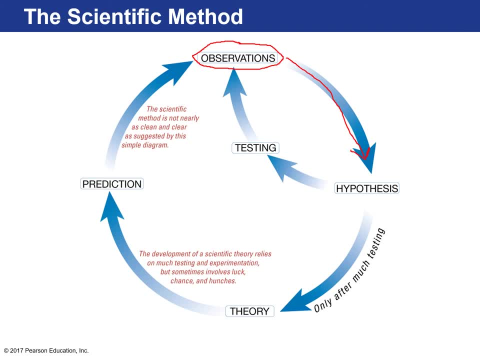 Are they trying to smack parasites off? Do they breach because they're back, or something right? And this is something that scientists have kind of been asking And they did a lot of research and testing and that's this process: to test whether or not their explanations for that behavior are right or wrong. okay, 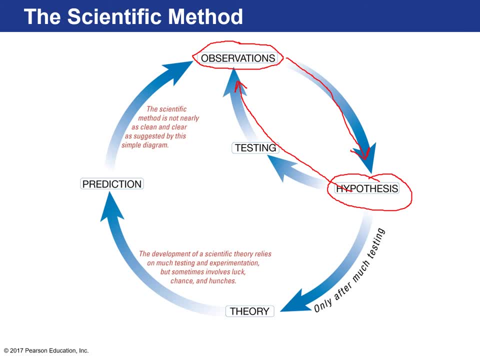 And so what scientists have done, after studying weeks and weeks of different pods of whales breaching and collecting data on that behavior, is that the whales actually use breaching as a form of communication. So when pods are kind of close together, they'll do that fin slapping. 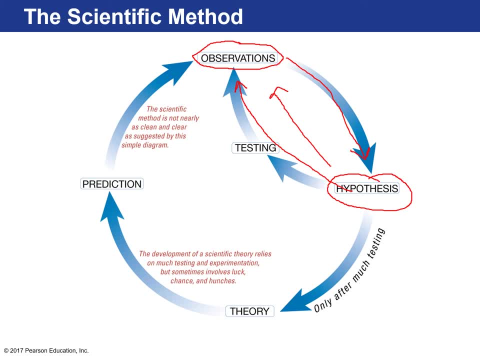 Their caudal fin, they'll bring it out of the water and then slap, And so that's how they can kind of make noise and communicate with pods that are close together. But if the pods are very far apart or there's a lot of noise in the ocean, like ships or something like that, 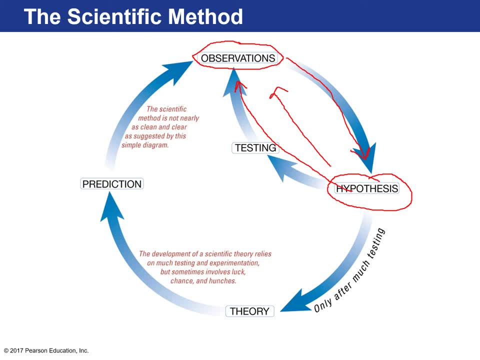 then they'll breach, Because breaching, you know, they're taking their giant bodies out of the water and then they're smacking down The water really hard like a hammer, and that makes a louder noise so that they're able to communicate over longer distances. okay, 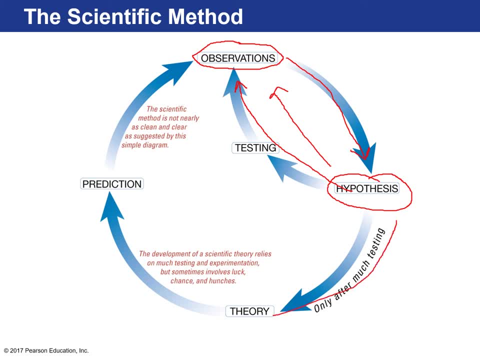 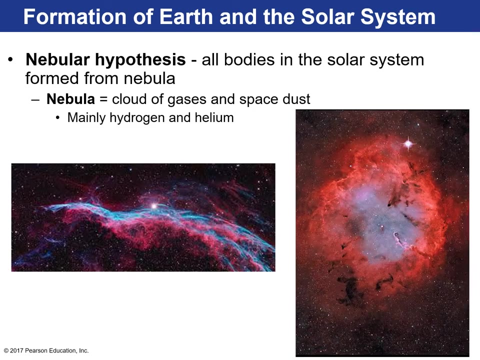 So only after a lot of testing do you have a theory? okay, And then perhaps we'll call that the whale breaching theory. okay, Then you can use those theories to kind of predict, perhaps, future observations. okay, All right, so let's talk about the formation of Earth and our solar system. 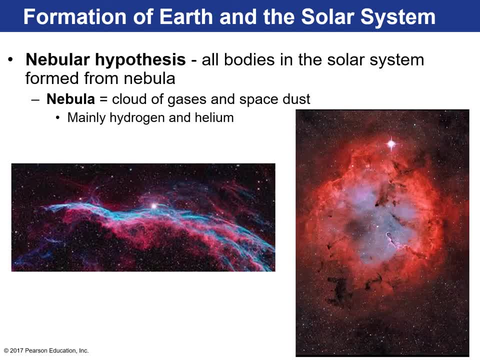 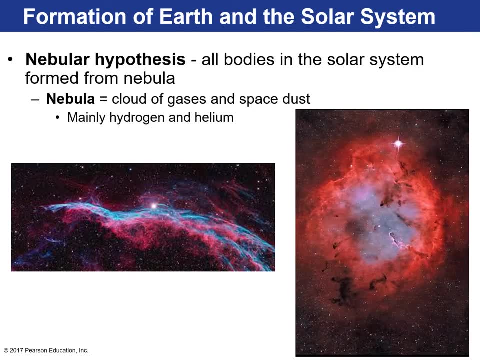 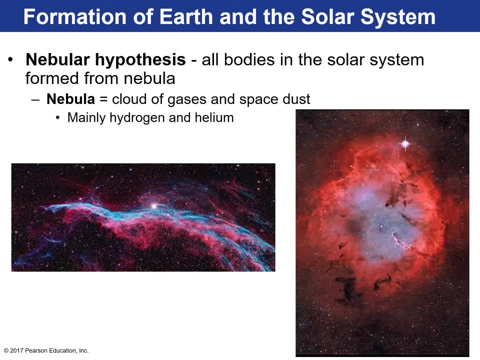 The nebular hypothesis. This is a hypothesis that all bodies in the solar system formed from a nebula and that's a cloud of gases and space dust. Space dust meaning like material like silicate material, rock material, metals and gas kind of in this giant gaseous three-dimensional nebula like you see there. 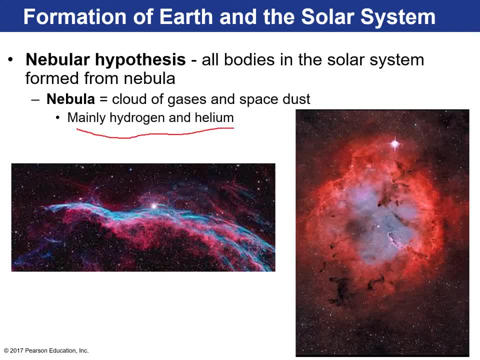 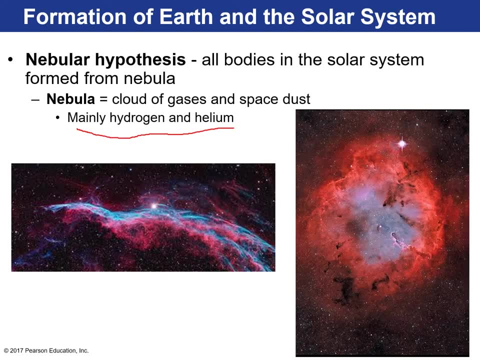 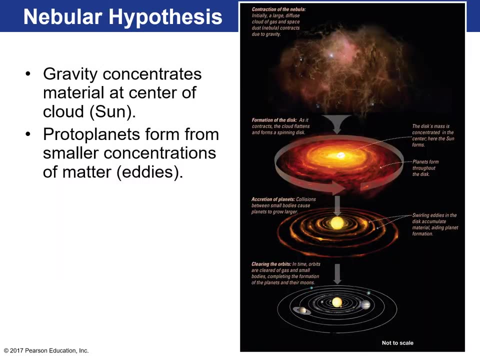 The composition of this nebula was mostly hydrogen and helium. okay, But as everything Kind of in this gaseous nebula has mass, it exerts a force of gravity. things start kind of contracting to one another. The center of the nebula is the protosun, or the protosun begins to form. 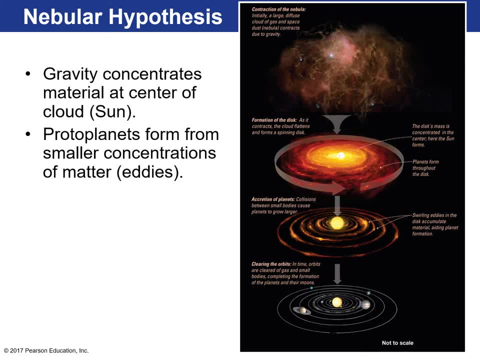 So essentially, gravity concentrates a lot of the material at the center of the nebula and the cloud starts to kind of collapse into the form of a disk and then it begins to rotate And as it rotates it kind of induces more collisions. 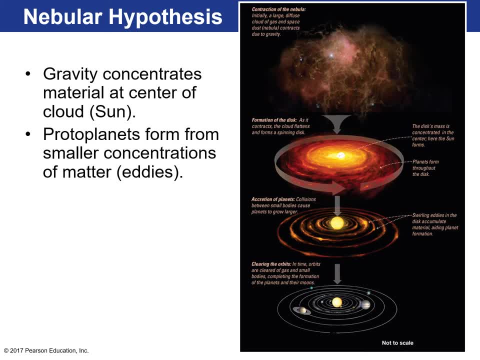 This mass material. you know a lot of that dust, a lot of the gas and surrounding the largest mass in this disk are protoplanets, including Earth. So Mercury, Venus, Earth and Mars are kind of the interior rocky planets. 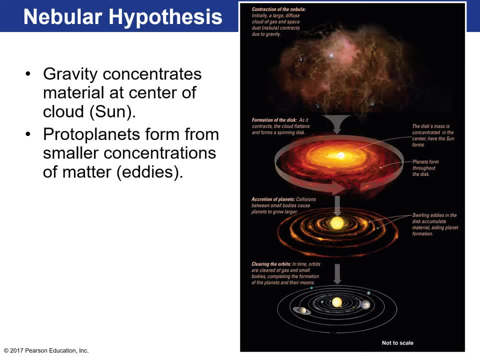 They're rocky because they're closer to the Sun and the heavier materials that coalesce to form the proto planets closer to the Sun. the Sun was hotter, so the heavier materials condensed closer to the Sun and then the volatiles, or the gases. those condensed 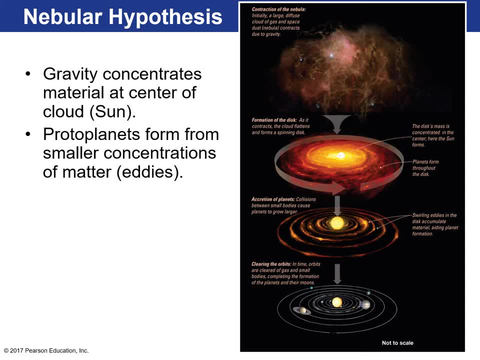 further away from the Sun, where it was cooler, it kind of formed ice and that's why, beyond Mars and the asteroid belt, you'll find the gas giants. okay, so this started to rotate and started to form our very first planet, as well as our proto Sun. okay, 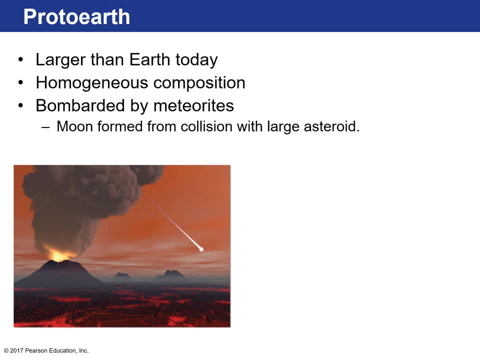 and our proto Earth formed. and initially as it formed, it was kind of a really hot kind of silicate rocky Earth that was kind of like a magmatic ocean and just slowly started to cool down. it was a lot larger than the earth today. it's kind. 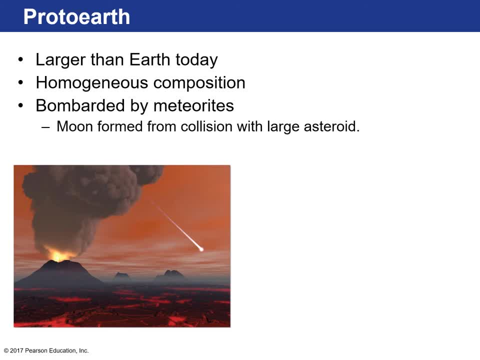 composition was homogeneous, meaning that it was kind of all one composition very well mixed, and it was bombarded by meteorites, and meteorites are just kind of leftover portions of Planetesimals that you know weren't part of planets. So there was a lot of collisions and that kind of really heated up the earth. 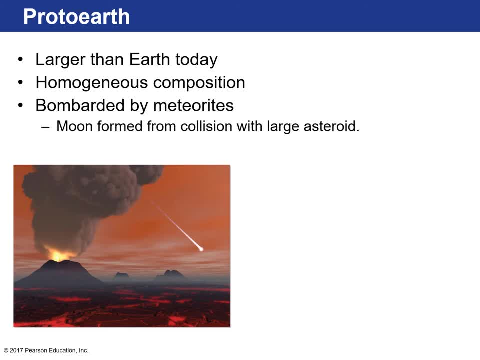 one planetesimal That was much smaller than the earth, was also kind of orbiting the Sun, but it was under the direct path of the of our earth and It struck our earth right and that collision kind of added a lot of material to our earth. and then the 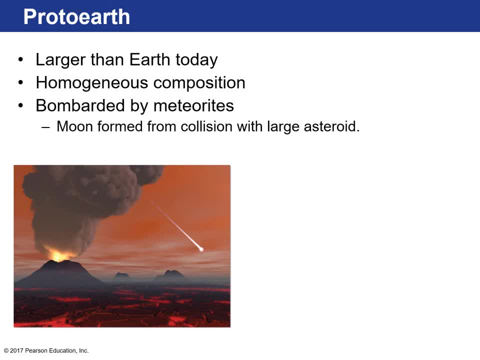 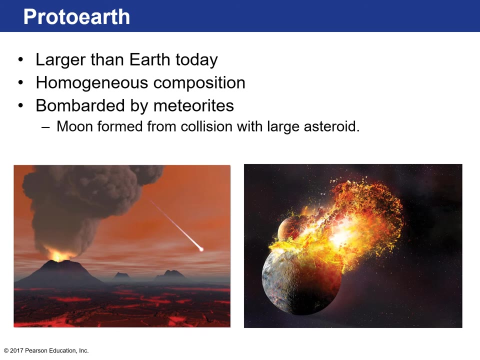 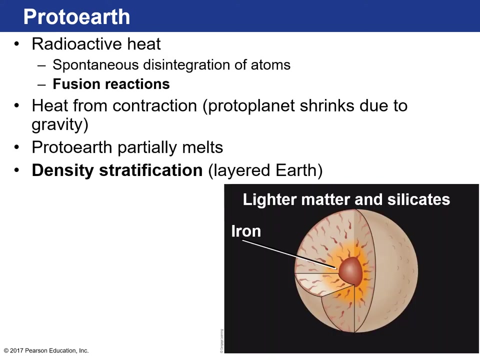 Rest of the material got caught in Earth's orbit and that became our moon. Okay, so our moons origin story essentially is a collision course with Earth. Boom, there you go, and there's an artist rendition of what happened. And then A lot of the lighter material, or lighter elements started to kind of float. 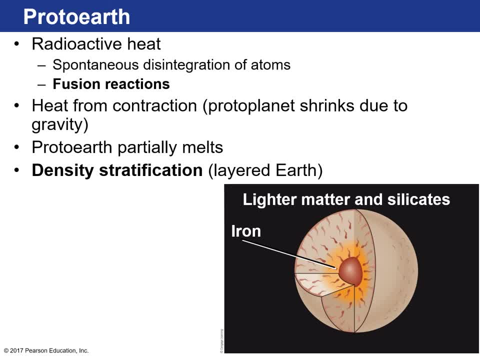 Towards the outer edges of the earth, kind of from the interior, a lot of the denser material like iron and nickel, Because it's heavier and denser and when you heat something like that up it sinks towards the center. It's like if you boil milk right. 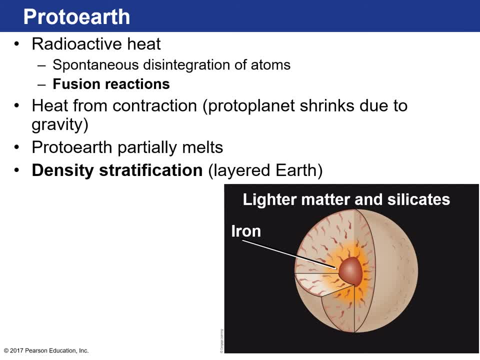 You boil milk, the cream rises to the top. That's the lighter material. So the light, you know, oxygen, silicon, potassium, a Lot of the lighter elements- started to kind of rise up, Okay, and this led to what we call the density stratification of our earth. 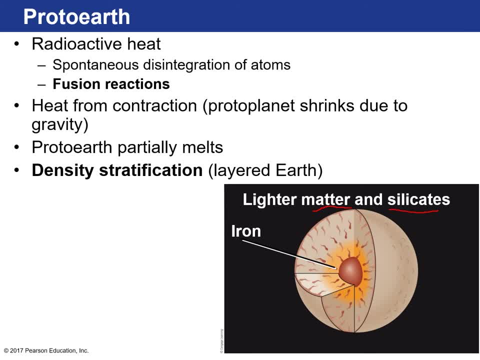 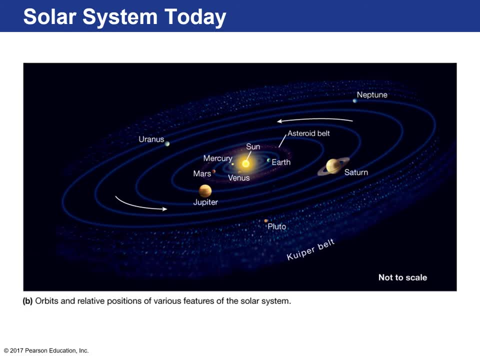 meaning Now the earth was becoming heterogeneous, meaning there that it was forming distinct chemical layers on our earth. Okay, All right, there we go. and here's our solar system Today. there's our Sun, for interior Rocky planets, Here's the asteroid belt, and then beyond this, then you start having the cooler. 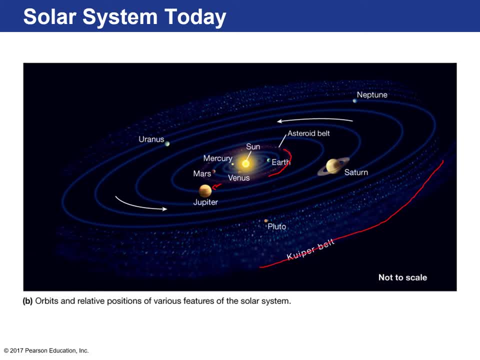 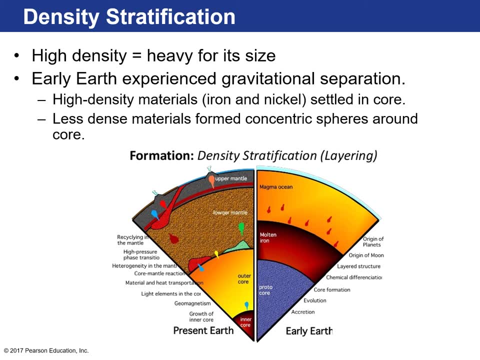 Gas giants right, and then here's the Kuiper belt- way out here. All right, so the density stratification here's showing you the different layers that formed early on in Earth's history, and this was a result of gravitational separation. So the high density materials like iron and nickel. 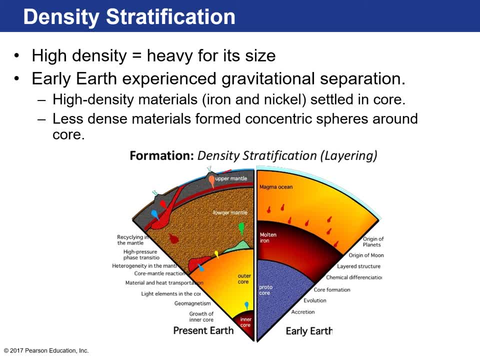 Settled into the core. okay, So here's the surface of the earth, All right. And then we have our, our crust and lithosphere. Here's the, the mantle portion of our Earth, and here's the outer course. All this here is made up of iron and nickel, very dense material sank towards the. 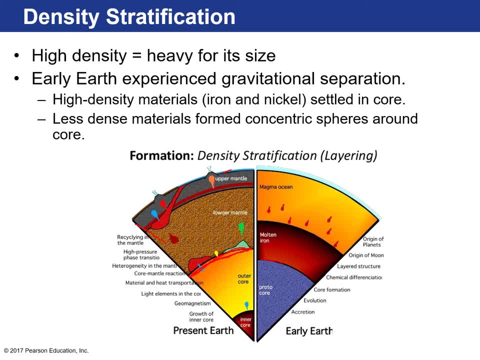 Center of our earth. So here's the distinction: early Earth. Here's the proto core, molten iron, and here's our magnetic ocean right. so this is very early on in Earth's history. this is the, the layers of our Earth today, and we'll go into this in more detail. so less dense. 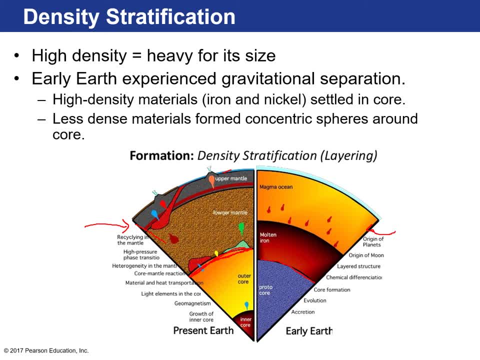 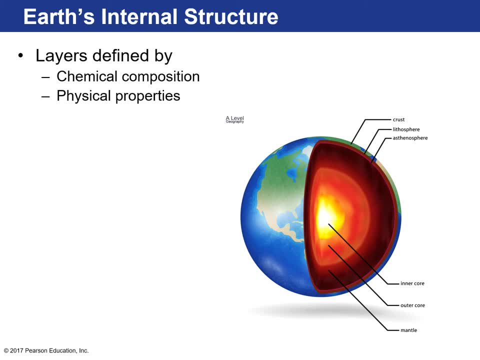 material formed spheres around the core. okay, so there's two ways we can identify the internal structure of our Earth. one is through the chemical composition and the others through physical properties. physical properties is essentially how the material behaves. so there's the lithosphere, asthenosphere, upper mantle, lower mantle and core. and if we're talking about chemical composition, 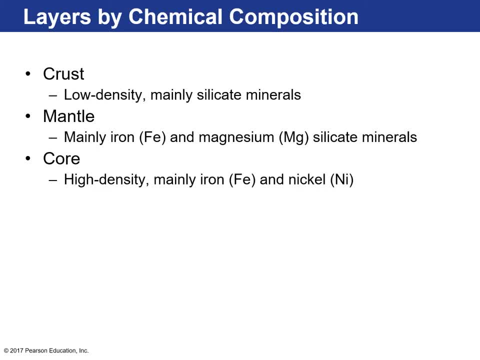 we've got the crust, mantle and core. I'll show you other pictures. so if we look at the layers of our Earth based on chemical composition, meaning like the different layers are differentiated by their chemistry, the outer and and kind of thinnest layers of our Earth are the layers that are 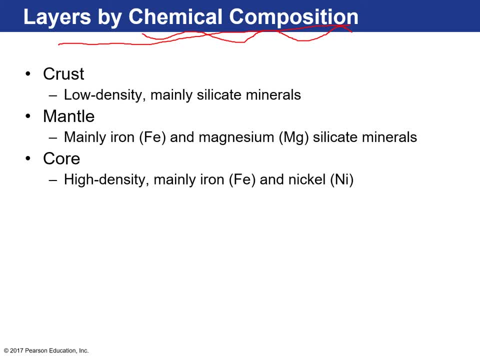 densest layer is the crust. that's a very low density. low density, mainly silicate rocks and silicate minerals. very light materials- silicon, oxygen, potassium, calcium- those are the typical light elements that you'd find in the crust. below the crust is the mantle. this is also rock silicate. 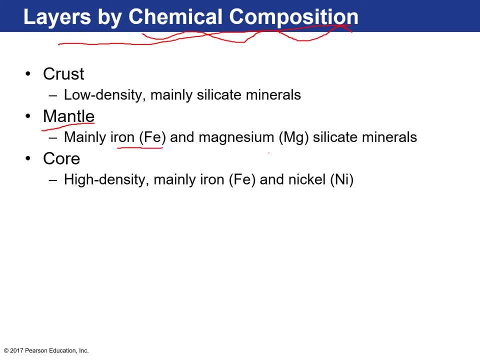 rock, but this silicate rock contains more iron and magnesium, and iron and magnesium are heavier. so that's the distinction between mantle and crust is that there's more iron and magnesium in these rocks versus the crustal rocks. and then when you get to the core, the kind of last layer, this is really made up of high density iron and nickel, and that's. 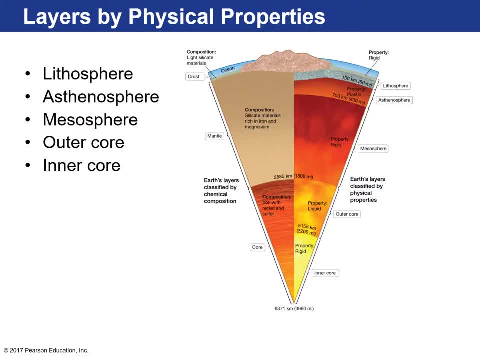 how it differentiates itself from the mantle and the crust. now, if we look at the Earth's layers based on the physical properties or how the material behaves, the outer layer is referred to as the lithosphere. the lithosphere is a material that is brittle. it is when it's under stress, right. that's why we have earthquakes and stuff like that. so it's very. 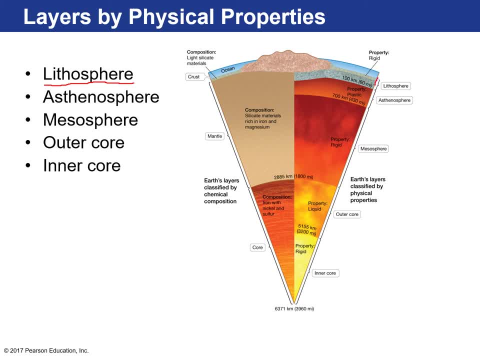 rigid and that's typically the upper 100 kilometers of the Earth. so from the surface, the bottoms of the oceans, or from the continents- so it's the crust plus the upper portion of the mantle- is considered the lithosphere, all right, so on average is about 100 kilometers, so that's the lithosphere. 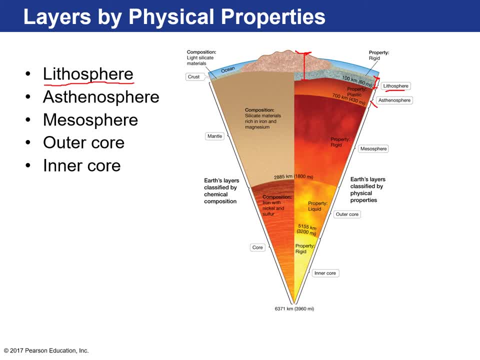 right here, all right below. that is the asthenosphere and that's exclusively in the mantle. now, the reason it has its own kind of distinguishing layers because it behaves differently. the asthenosphere is hot, the rocks are very close to their melting temperatures, so that makes it very weak and that 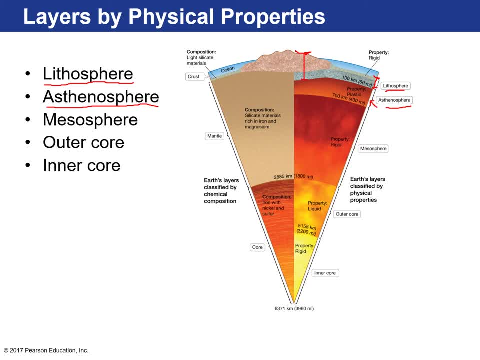 stuff is plastic and can move around okay, and so essentially that creates a division between the lithosphere and the asthenosphere, and lithosphere can kind of float on top of the asthenosphere. then as you go deeper and deeper within the Earth you run into the mesosphere, which is this area, right? 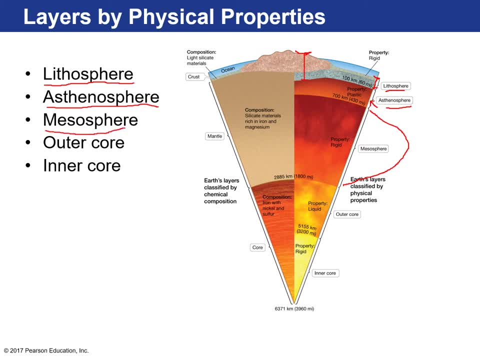 here and that's also in the mantle. so it's just mantle rock, but it becomes more rigid, and the reason why it becomes more rigid is because of the increase in pressure. okay, then, once the mesosphere is over, you get to the outer core, and the outer core is kind of its own distinct, distinct layer, because it's actually liquid. this 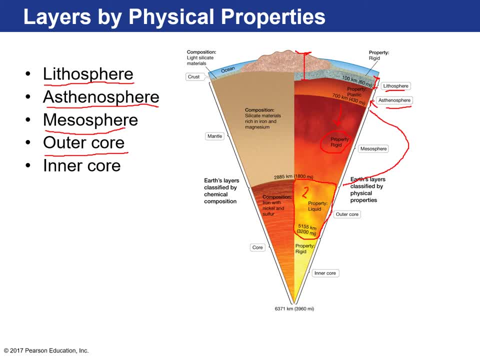 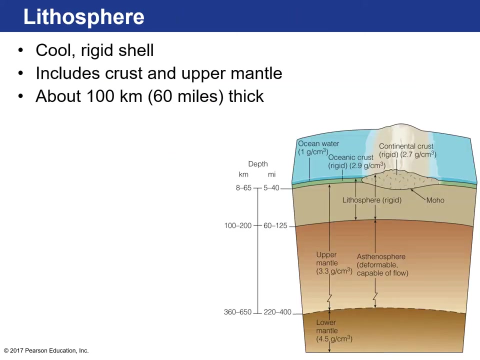 is liquid iron and it kind of moves and convects, okay. so this is the outer core- liquid iron- and then the inner sphere here, um, the iron. because of the increase in pressure, the iron actually solidifies and this is a solid. so the inner core is solid. okay, so these are the layers based on how the material behaves. all right, just. 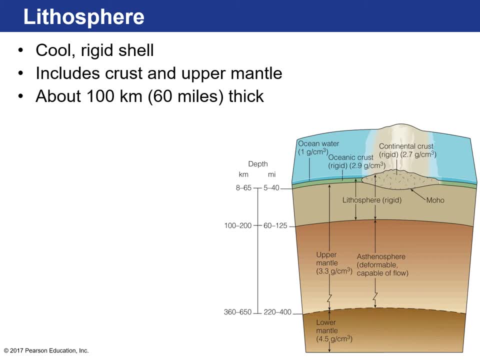 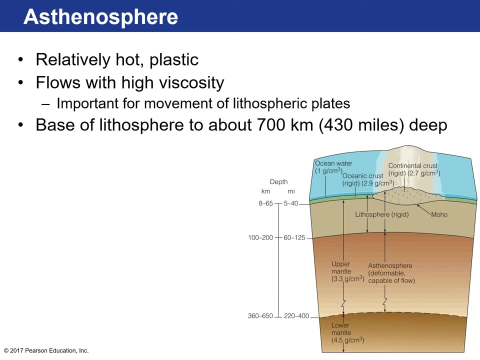 to reiterate, here's the lithosphere: cool, rigid shell surrounding the Earth, on average 60 miles thick, includes the crust and upper mantle. okay, so here's the upper mantle. this is the lithosphere: ocean crust and continental crust plus upper mantle. all right, then they've seen a sphere: hot plastic mantle material. that's this area here. 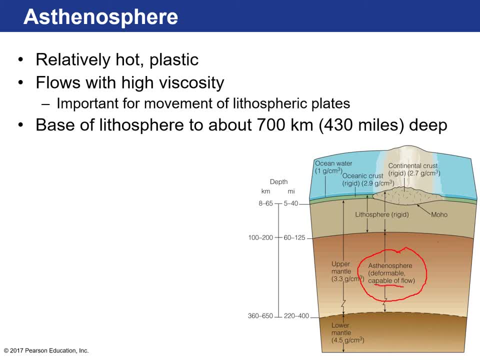 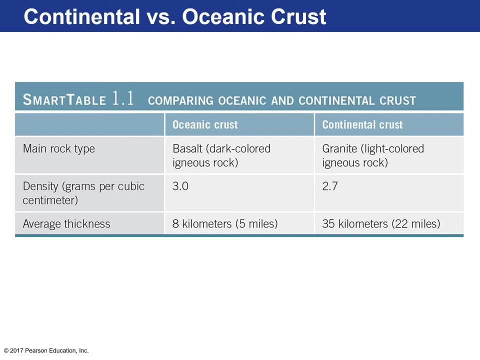 it's deformable, capable of flowing, because it's very weak, okay, and that goes from the base of the lithosphere to about 430 miles below that, so the pretty prominent layer. um, there's two different types of crust: there's continental crust and there's ocean crust. 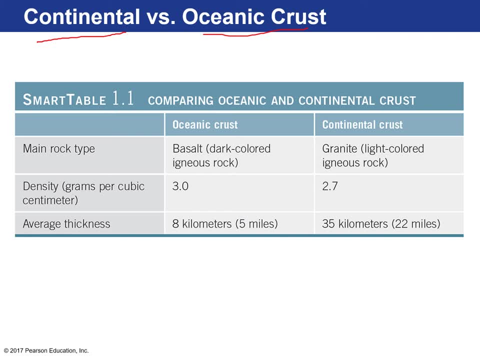 um, the rock that makes up a continental crust is granite, right? so think of your countertops in your kitchen. that's granite. that's an igneous rock, or a rock that formed through the cooling of magma. basalts also forms from the cooling of lava on the surface of the Earth, but basalt makes up the ocean crust, so 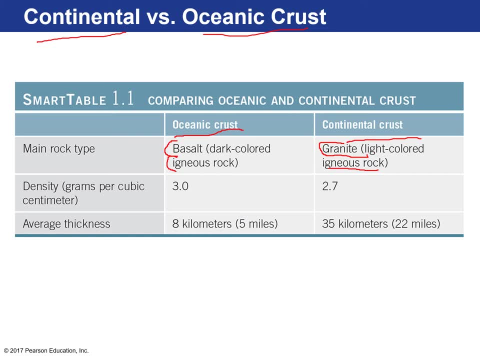 if you go out into the oceans, go to the bottom of the ocean, the sea floor, get through all the sediment, you're going to run through a bunch of basalt and this is a volcanic rock and it's uh, kind of black in color, okay, and the main difference is that basaltic rock is a lot denser, meaning it's. 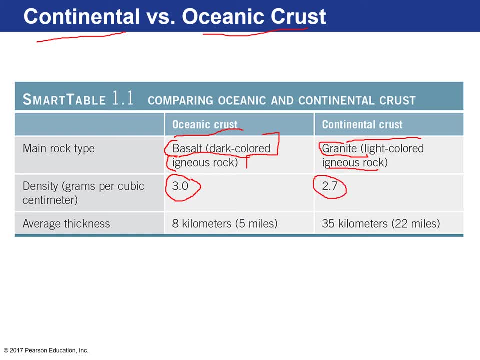 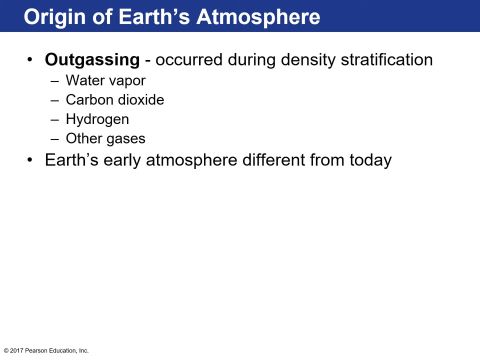 heavier than granite. okay, so when you're talking about the ocean crust, the ocean crustal thickness is about five miles, while on continents, on average is about 22 miles. there's a big difference there. all right, what's the origin of our atmosphere? well, uh, it formed through outgassing. that's a process where carbon dioxide, water vapor, hydrogen 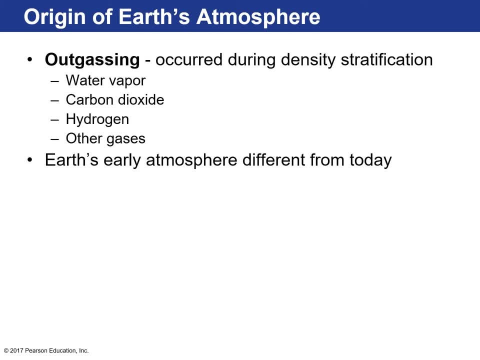 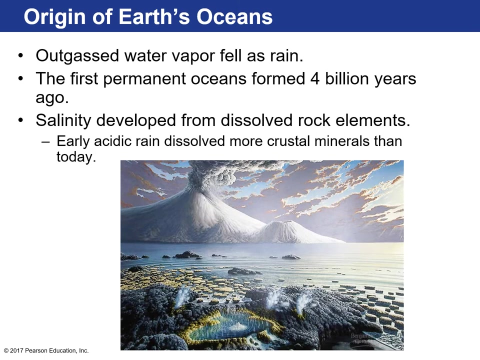 sulfur dioxide. other gases are expelled from fumaroles or volcanic vents or hydrothermal activity at the bottom of the ocean. um, this is where our atmosphere originally came from, and our early atmosphere, different from our atmosphere today, didn't have any free oxygen. so as these volcanic eruptions kind of delivered gas into the atmosphere, obviously got caught. 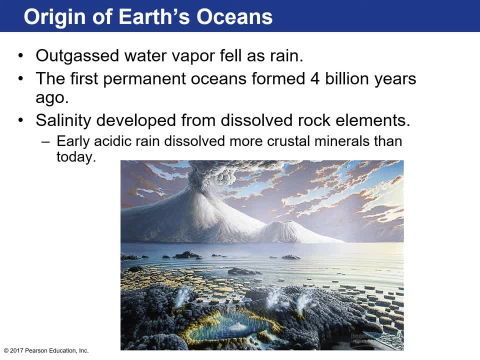 by Earth's gravity and then kind of trapped there a lot of the water- water vapor- that was coming out of it as a gas condensed in the upper atmosphere and fell back as rain, and that's what formed our first kind of pooling water in the low areas of our early Earth. okay, and permanent oceans formed as a result of. 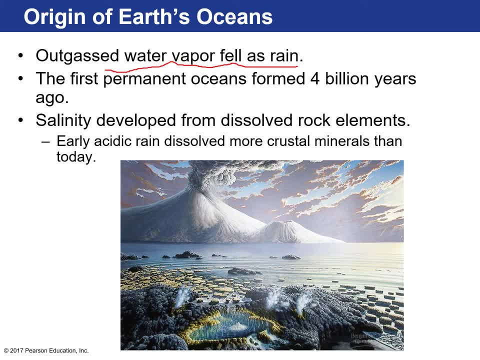 this repeated process about four billion years ago. the reason why the oceans salty is because that rainwater dissolved the exposed rocks and the kind of weathering of the exposed rocks brought a lot of the dissolved solids into the water, and that's what makes it salty. you 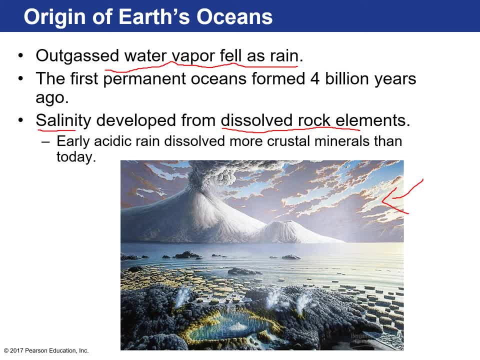 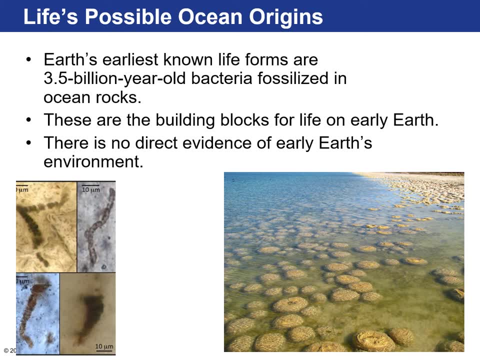 okay, so this is an artist rendition of what early Earth would have looked like. life showed up. the Earth formation was about 4.5 billion years old, and the oldest evidence of life on Earth that's fossilized are these stromatolites. these are bacteria that lived in shallow parts of the ocean right here they lived in. 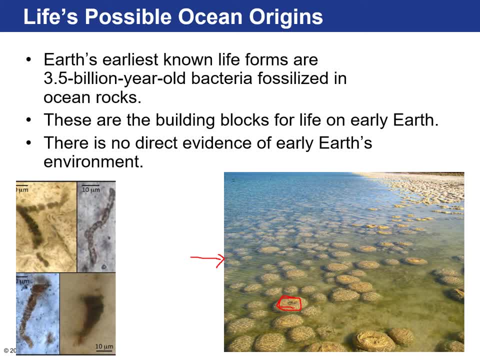 kind of bacterial mats and created these mounds and these are fossilized and a lot of rocks. this organism still exists today. you can find it in Australia- Sharks Bay, Australia- but essentially they live in these shallow waters and they photosynthesize. okay. so there, the there. 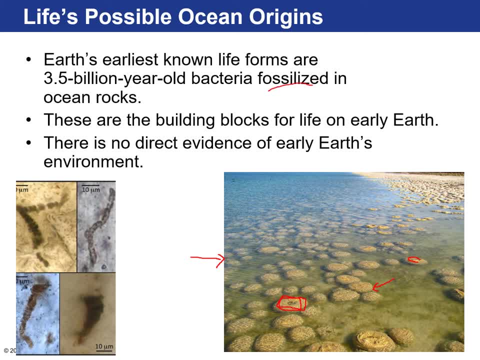 these fossilized organisms that lived on earth 3.5 billion years ago- single cell bacteria, but earlier than that there was other. there's other evidence of birds burrowing organisms, but scientists think that even earlier than this, about 500 million years before, stromatolites showed up in the fossil record there. 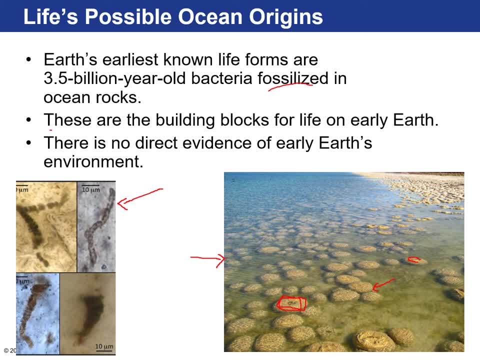 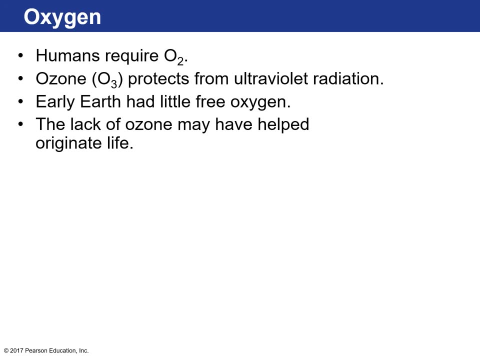 must have been Archean bacteria that existed in kind of really inhospitable environments like hydrothermal vents at the bottom of the ocean. It was likely a starting place for a lot of organisms. Okay, oxygen kind of showed up much later. It was a major oxygenation event. Humans require oxygen. Try to go. 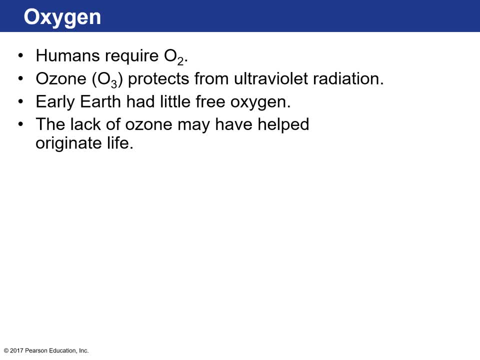 without some for a few minutes. It's terrible, But the reason why oxygen started to show up in our atmosphere is because of photosynthesizing organisms, kind of like those stromatolites in the ocean. They're the one of the. 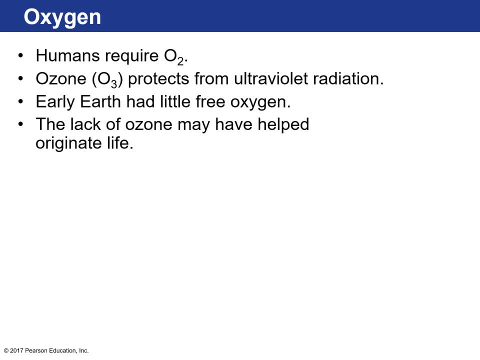 first organisms that evolved to undergo this process of photosynthesis, where they convert carbon dioxide and they excrete oxygen as a waste product and create carbohydrates that they use for food or sugars, And so that process of photosynthesis created a lot of free oxygen and, initially, all the free oxygen. 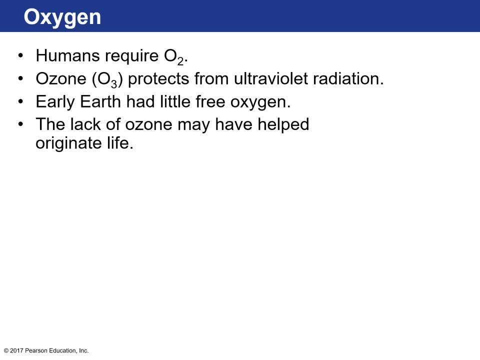 would react immediately with iron in the ocean and then deposited out as sediment. so it took about like 1.2 billion years of organisms on Earth consistently photosynthesizing to actually start to change the composition of the atmosphere. and once free oxygen started to form in the atmosphere, ozone began to form in. 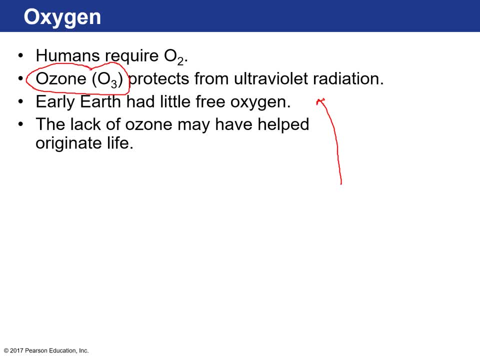 the upper atmosphere and that was a huge step for evolution of early organisms, because the ozone layer will filter out a lot of UV radiation and if there's less UV radiation striking the surface of the earth, then that allows for kind of organisms, single-celled organisms, that proliferate and even evolve into. 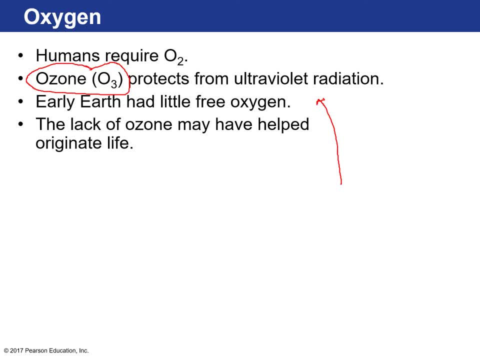 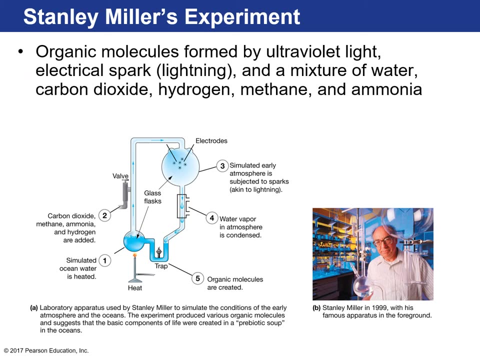 multicellular organisms. okay, in the beginning we didn't have an ozone layer, so a lot of the organisms that we saw in the upper atmosphere were actually organisms, especially the anaerobic bacteria, which require little oxygen, may have helped originate life. in fact, this guy, Stanley Miller, he's a scientist who 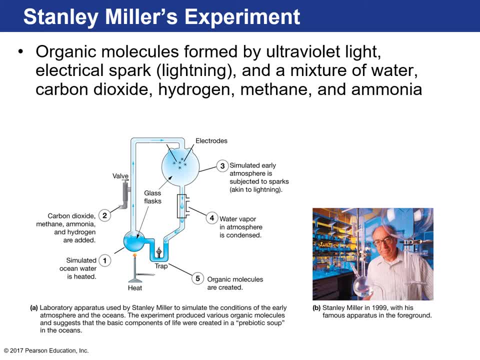 as a graduate student came up with his experiment where he kind of simulated Earth's early atmosphere. okay, then added some electrodes to signify like kind of like lightning strikes, and so that mixture was carbon dioxide, hydrogen, methane and ammonia- something you typically see- and his kind of result of doing this experiment. 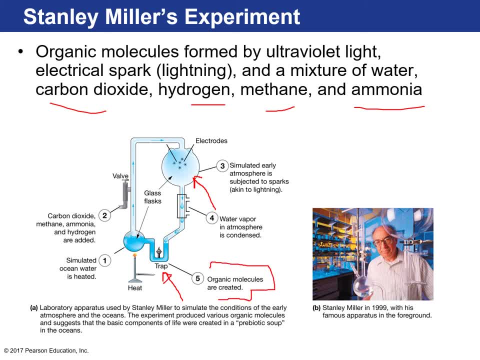 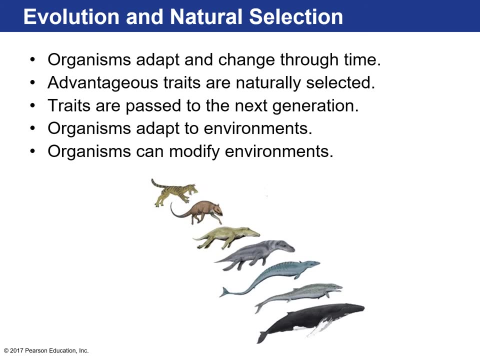 where organic molecules were created. so he kind of created something almost out of nothing and that's believed to be kind of like the conditions for how life began in early earth, kind of mimic, that pretty famous experiment. so what that led to, we had living things on earth, initially very simple, single-celled. 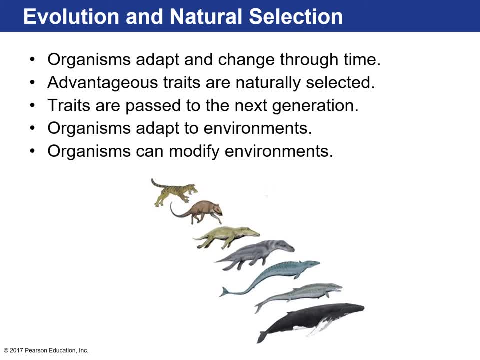 organisms. they evolved. they evolved, they changed and the organisms adapted to different environments. luckily the oceans are very well ubiquitous, but also an environment where there isn't much change in daily temperatures. it's a very kind of stable environment and that allowed for organisms to kind of proliferate in all areas of the ocean. but then they started to develop new organisms. that changing the climate is a big thing in the very early part of eternity and that allowed for organisms to kind of proliferate in all areas of the ocean. but then they started. 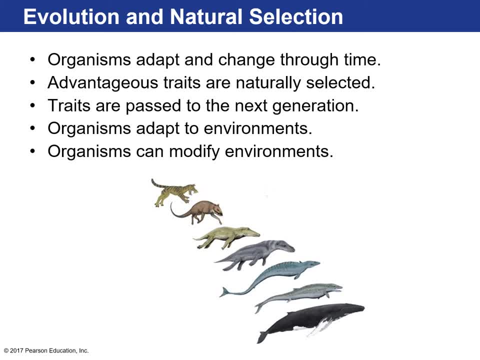 kind of proliferate in all areas of the ocean, but then they started to adapt and change to different environments, and so what happens with evolution is organisms that just so happened to have advantageous traits, which could happen just through genetic variability or some sort of fortunate mutation. they're 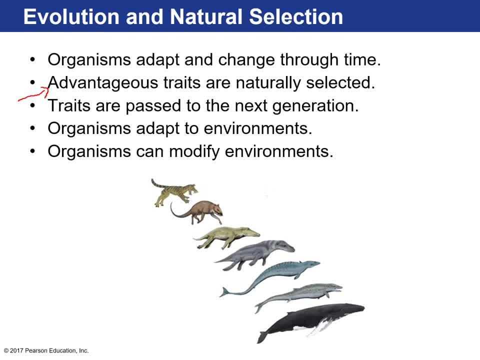 quote-unquote- naturally selected, meaning that, for whatever reason, that trait might help them survive better, and then they can pass that trait on to their offspring, and then they're that offspring can proliferate, and so on and so forth. so those traits are passed on to the next generation, and then they become 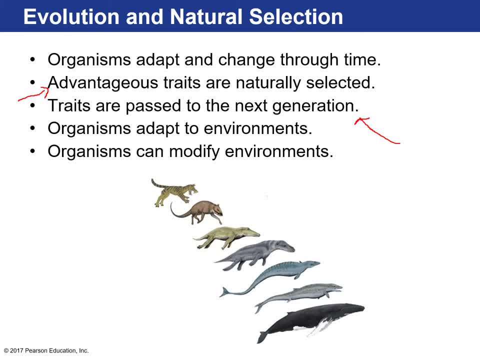 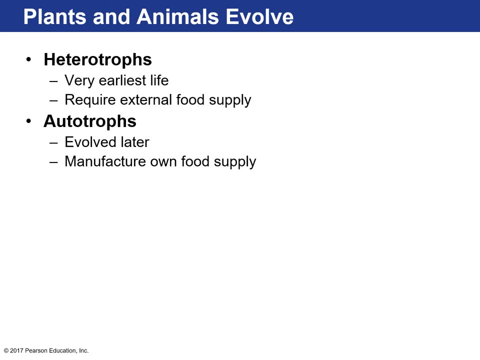 more successful, and that's how organisms adapt to environments and then eventually, once the organisms become so abundant and proliferate, they can actually modify their environments. okay, so that's how evolution and natural selection work. heterotrophs are kind of the very earliest form of life. okay, they require 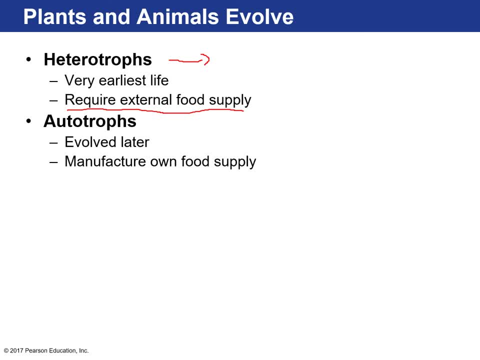 an external food supply, meaning like they need to like bump into other things to kind of consume food later on. autotrophs evolved later which are organisms that manufacture their own food. think of those stromatolites building those mounds and photosynthesizing, the process of 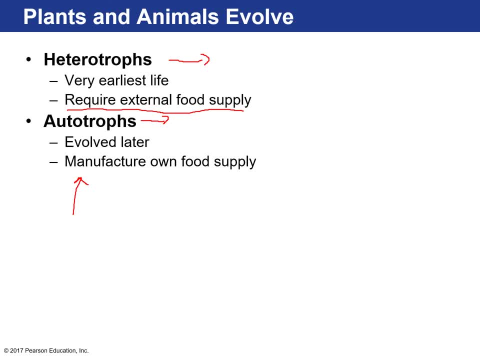 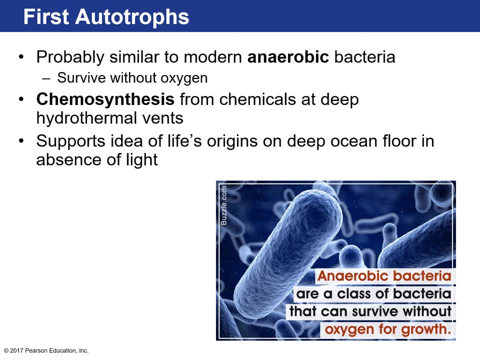 photosynthesis is manufacturing your own food supply. they don't need anybody else, right? so the first autotrophs to form were very similar to anaerobic bacteria. these organisms live in environments with very little free oxygen. okay, so today's day and age, I mean in deep underground or in 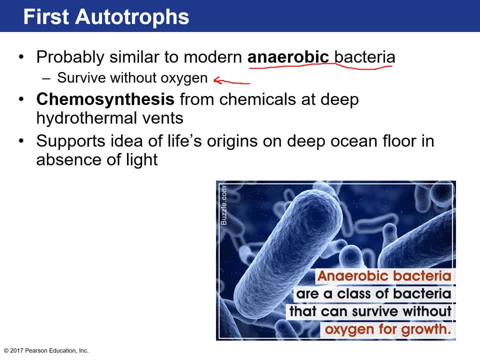 environments that are with very little oxygen, kind of unusual environments. we still see them today, but they actually- some have evolved to generate their own food, kind of like photosynthesis, but they don't require the Sun. it's called chemosynthesis and they actually use chemicals from volcanic or hydrothermal. 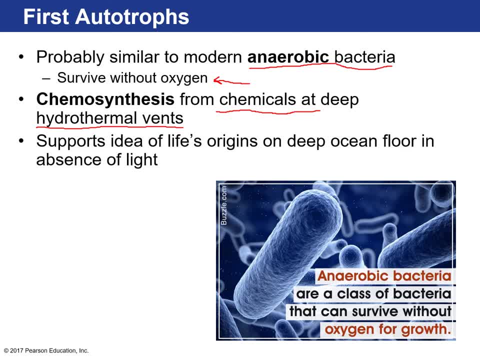 vents to create sugars to manufacture their own food. so once we discovered this, by the way, which we only discovered- these organisms in the 1970s that supported the idea that perhaps the origin of life on earth were was through these anaerobic bacteria, in these kind of hydrothermal vents at the bottom of 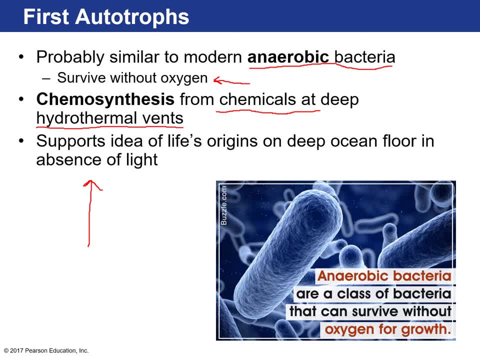 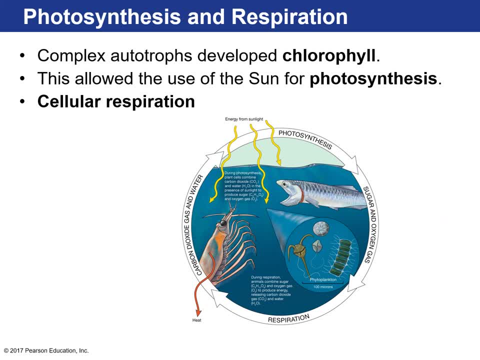 oceans, because that's a likely environment that would have existed four billion years ago. those are the first, and then, later on, organisms kind of evolved to be more complex. eukaryotes showed up, which are single-celled organisms that have a nucleus and a bunch of different organelles that 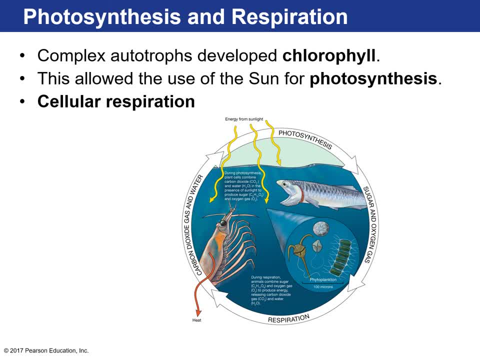 perform different functions. then that evolved to multicellular organisms, and then there's- I mean well, photosynthesis was occurring before then, but those complex autotrophs developed chlorophyll and that allowed the use of the Sun for photosynthesis and created this process of photosynthesis to create sugar and 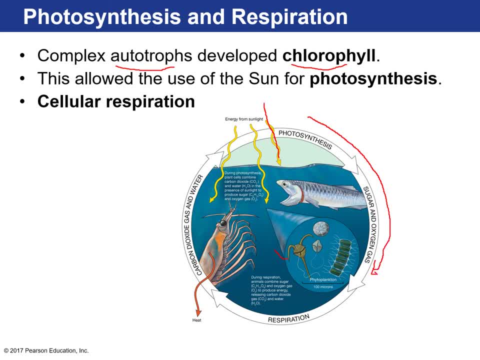 excrete oxygen gas and put that dissolved oxygen in the water to allow for other organisms to replicate the oxygen that was in the water and that was then produced to aspirate right other organisms in the ocean. when they move through the water they're able to use that dissolved oxygen to breathe. 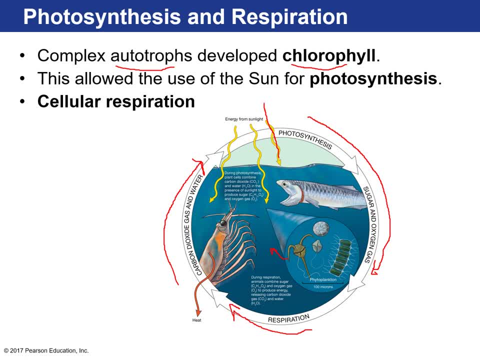 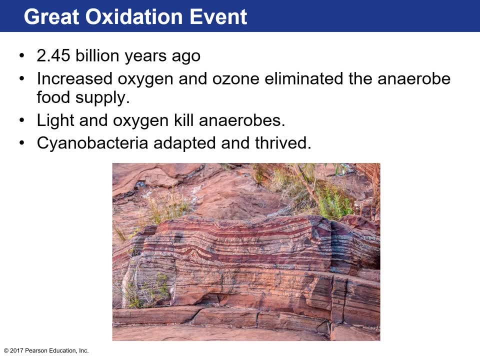 right, and then they excrete carbon dioxide and gas into the water, and then that carbon dioxide is used up again by these small autotrophic organisms here. okay, so after the formation of kind of, or the arrival of, stromatolites in the, the atmosphere took about a billion years of this occurring on Earth to increase the. 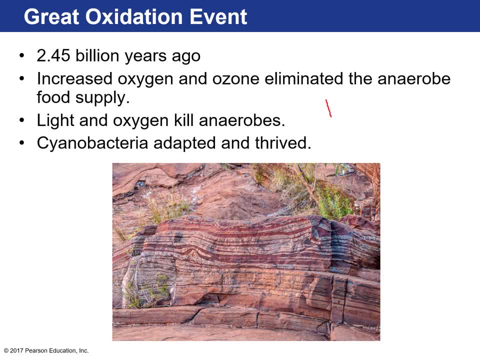 oxygen so much that oxygen was present in the atmosphere and formed an ozone layer. And the reason why we know this is because there are these deposits called banded iron formations. You can see this here. These are deposits of iron at the bottom of the ocean, and the reason why these deposits 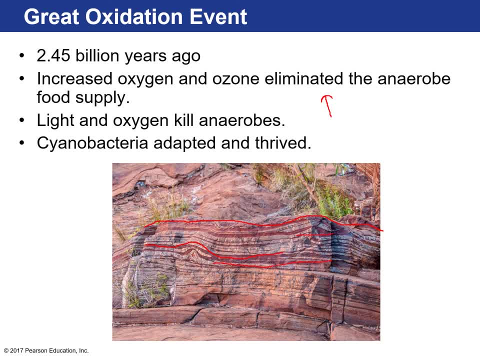 are here is because all the free oxygen that was pumped into the ocean would immediately be used up into the sediment and deposited, All the free oxygen. But as soon as enough oxygen was being used up and not bonding with iron in the water, then it could go into the atmosphere and these deposits no longer exist. 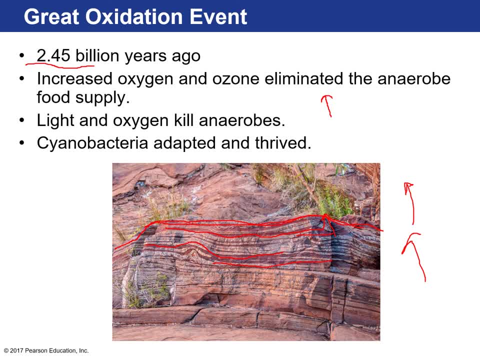 So these deposits stopped. This is about 2.5 billion years ago, or that's the youngest deposit we can find of banded iron formation. This is a typical iron ore that we mine And sadly, what happens? a lot in Earth as the environment changes. there's major mass extinctions. 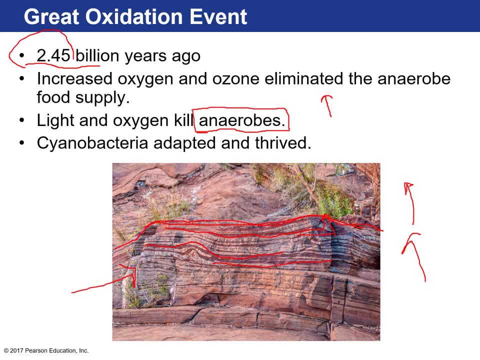 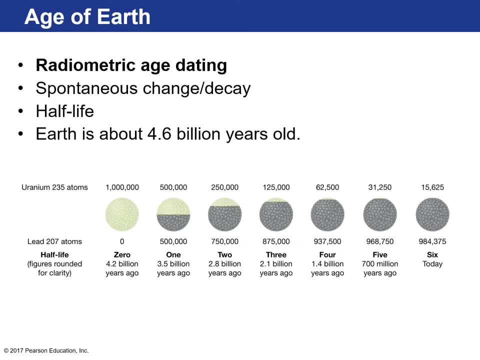 the anaerobic bacteria now, with all this free oxygen in the atmosphere, had fewer and fewer environments to live in, so they kind of died off. The Earth is 4.6 billion years old And we know this because This is the product of radiometric age dating okay. 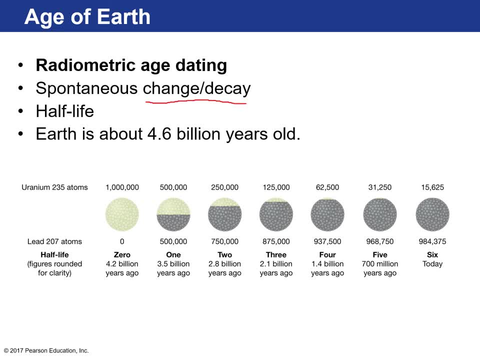 That's the spontaneous decay of radioactive elements. alright, As one example is uranium 235. This atom is so large its nucleus is unstable, so it'll undergo radiometric decay and it'll spontaneously shoot out parts of its nucleus outwards and decay into a new element. 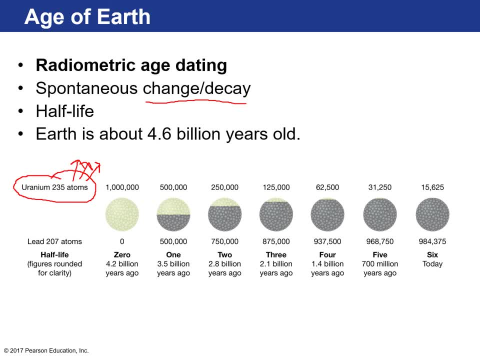 But it happens at a predictable rate. predictable rate and a rate that we can calculate. And if half of those atoms decay into its daughter isotope, which has led to O7, that's called one half-life. Okay, so if you have, 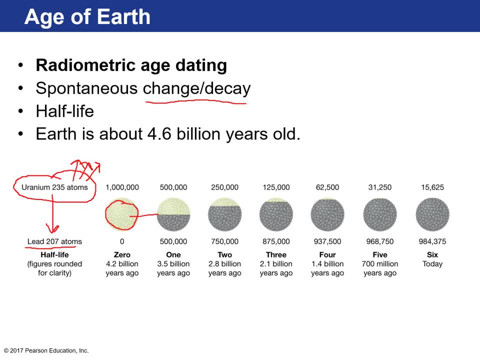 a million of these atoms here 4.2 billion years ago after one half-life. about 700 million years have gone by And you can keep doing this half-life game up until six half-lives, which is today, And so essentially you can age-date a lot of volcanic rocks. You can. 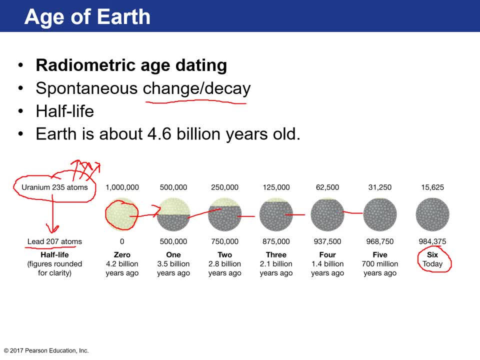 age-date meteorites. That's what we've done. We've age-dated a lot of the floating material that didn't coalesce into a proto-planet, that's part of the asteroid belt, and have landed on Earth. They all come up with the same date and that's 4.6 billion years, And so that's. 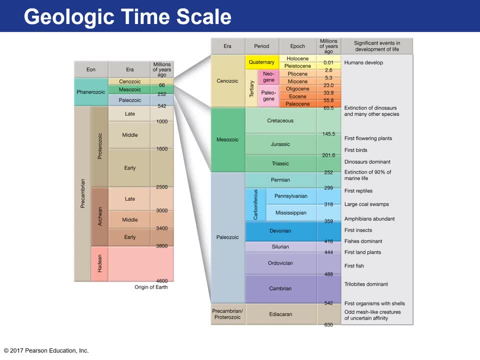 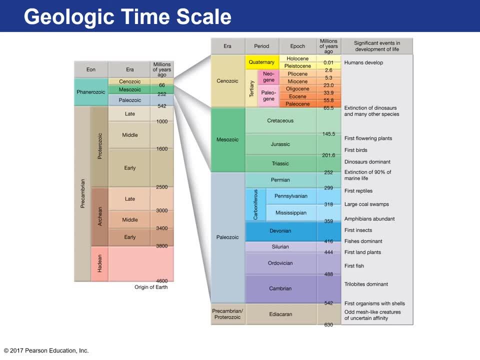 geologists over a long period of time, you know, through and also collecting fossils and putting rock units in terms of age relations, in terms of relative dating like what's older, what's younger, putting that in order And then, later on, assigning radiometric dates. 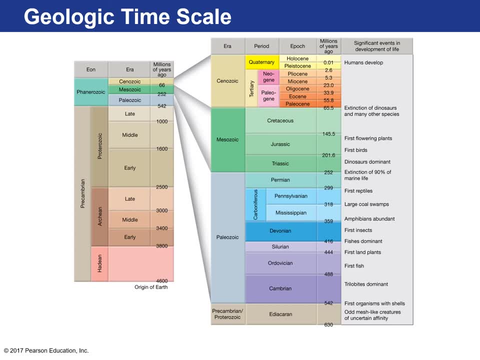 Here's the entire geologic timescale, from the origin of Earth 4.6 billion years ago to the first organisms with shells to show up in the fossil record 542 million years ago. right, so here's. here's the entire geologic time scale, to scale so most of about four billion years of. 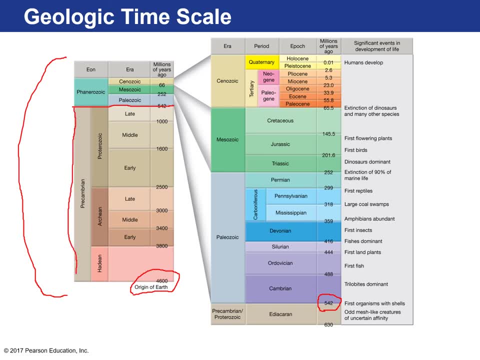 earth's history has been very, uh, simple. life forms, okay, uh, no fossil record whatsoever. all right, remember, uh, 3.5 billion years ago, right around here is when those photosynthesizing cyanobacteria showed up. but as far as the fossil record, nothing showed up until about 542 million years ago, and